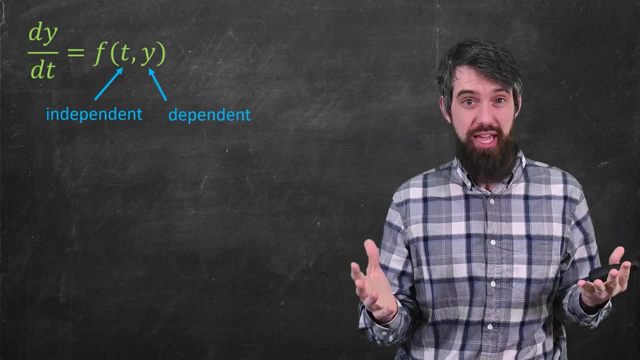 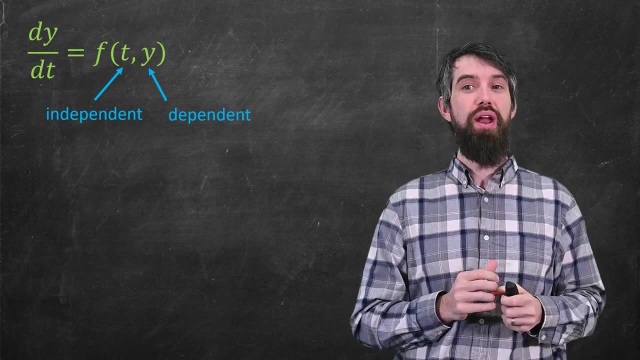 t, but t is just independent. So that's the generic case for a first-order differential equation. So what makes it autonomous? Well, an autonomous differential equation is one where the t just doesn't appear. I mean, it's still a derivative with respect to t and 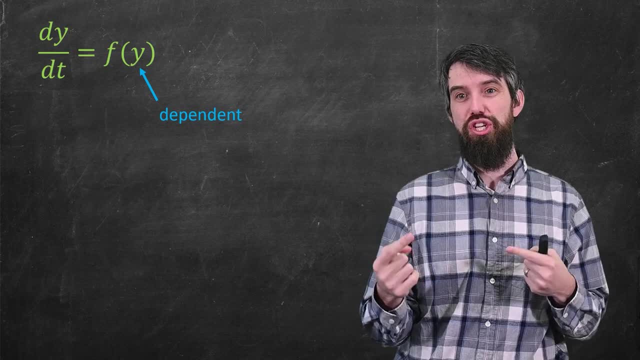 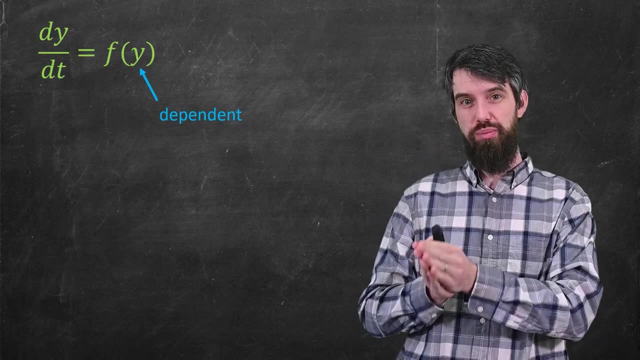 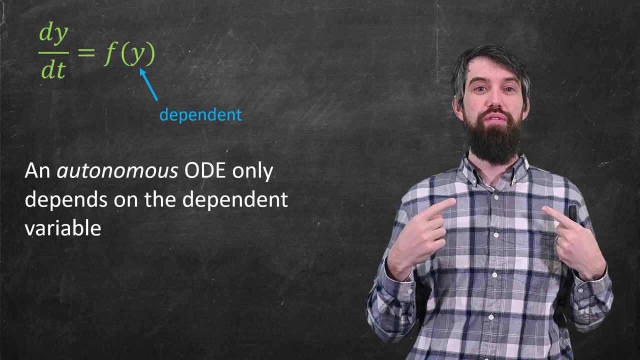 y still depends on t. But the explicit definition of the differential equation- it only depends on y, It's a derivative of y- is equal to just some expression in terms of y. So our definition is that an autonomous, ordinary differential equation is one where the derivative only depends explicitly on. 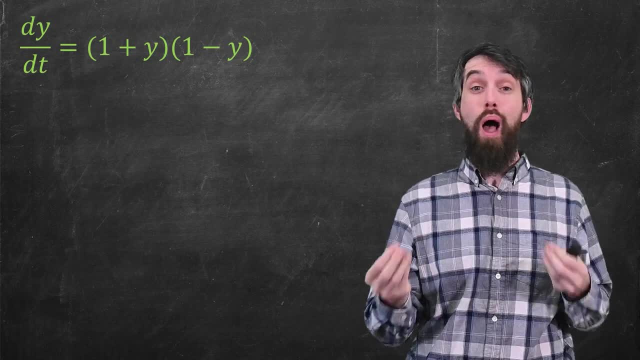 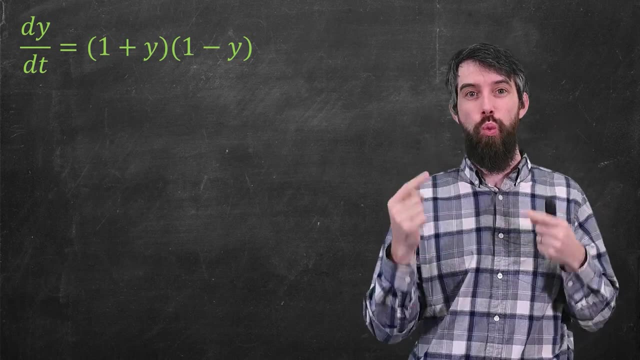 the dependent variable y. So here's an example. This is the derivative of y with respect to t is equal to 1 plus y times 1 minus y. That right-hand side only has y's in it. And one thing I want to note right off the bat is that if you were trying to figure out, 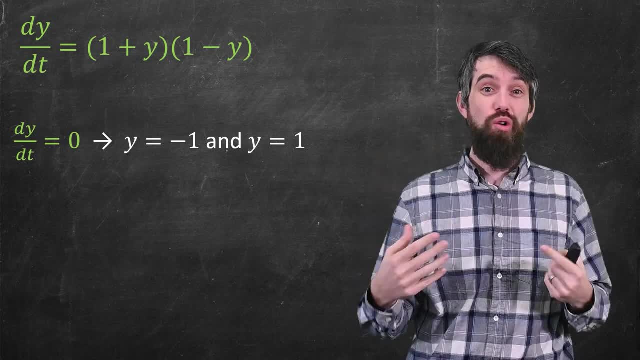 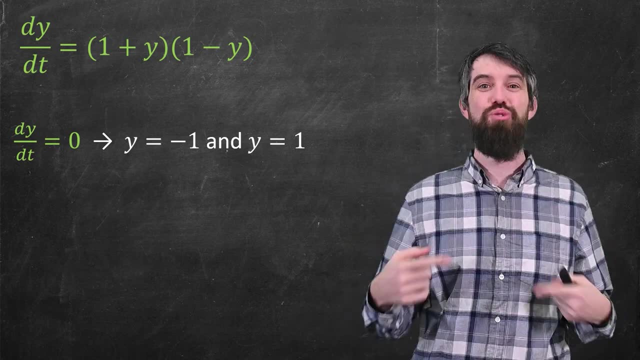 well, when is the derivative equal to 0, then you'd get that y is equal to minus 1 and y is equal to 1.. If you knew this was your derivative and you were in math 100, you'd say its critical. 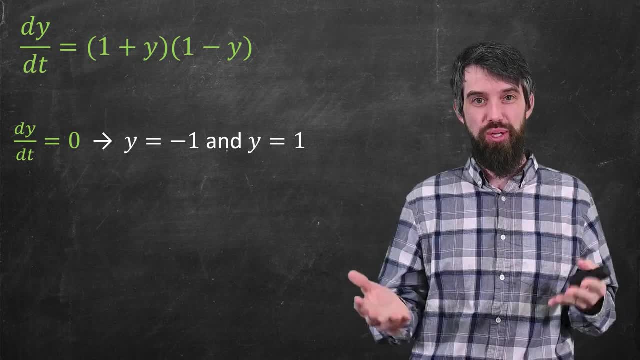 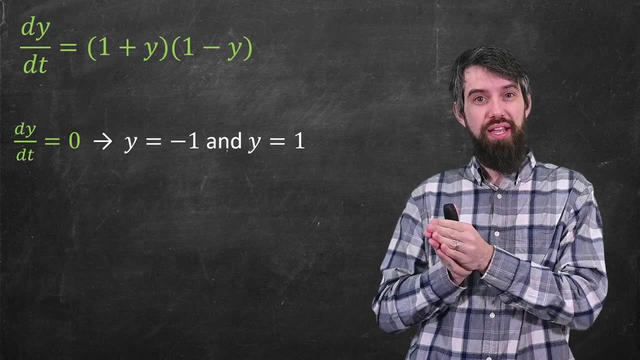 points were at minus 1 and 1, where the derivative was equal to 0.. So now we're going to turn to the computer to help us graph it, and I want you to keep these two spots- y equal to minus 1 and y equal to 1, in mind. So I'll open up my Jojoba to plot slope fields. 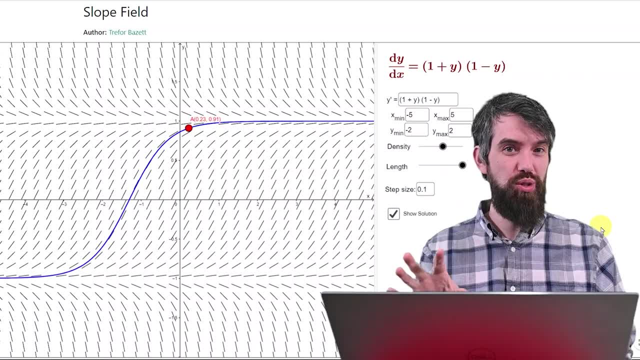 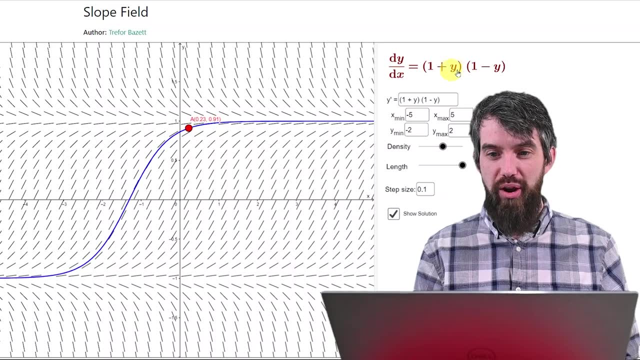 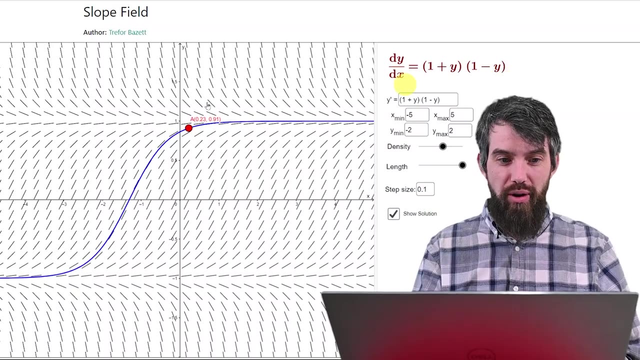 and I plugged in 1 plus y. 1 minus y is equal to y prime, And this is the kind of behavior that I get. So I want to notice a few things. First of all, recall that our two spots where the right-hand side was 0 was either y equal to 1 or y equal to minus 1.. And what you'll? 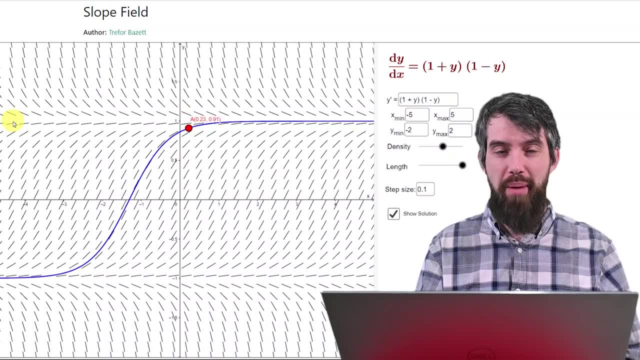 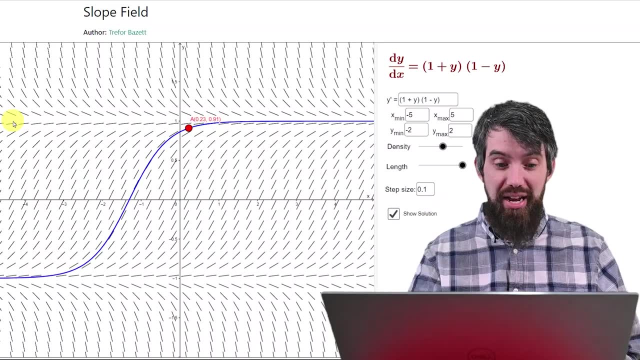 notice is if you go along the line y equal to 1 up here, it's where the derivative is 0. And if it plotted at that exact point you'd get horizontal lines, y is equal to minus 1.. That's down here. 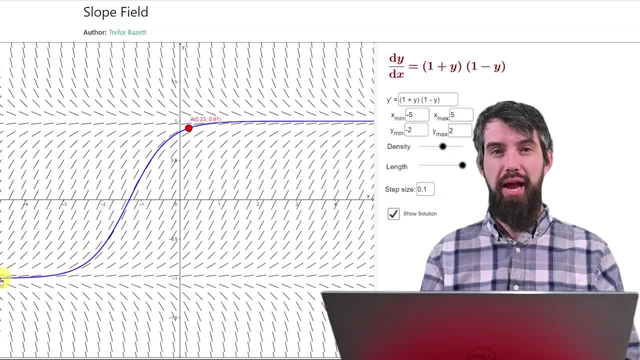 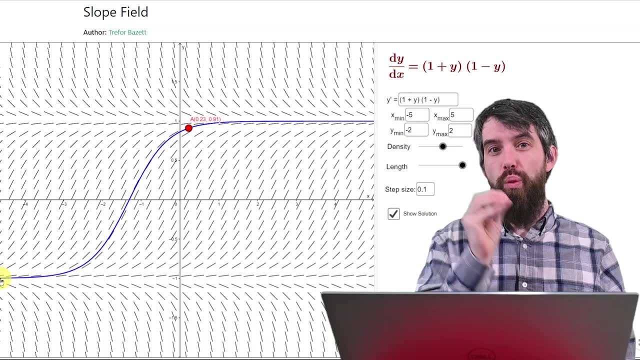 And minus 1, it's going to similarly be this horizontal line, And so these are what we call equilibrium solutions, And the idea of an equilibrium solution is: if you started at y equal to 1,, if your value is exactly y equal to 1, then the derivative would be: 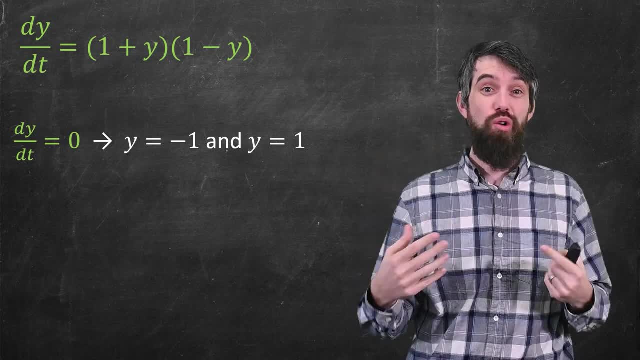 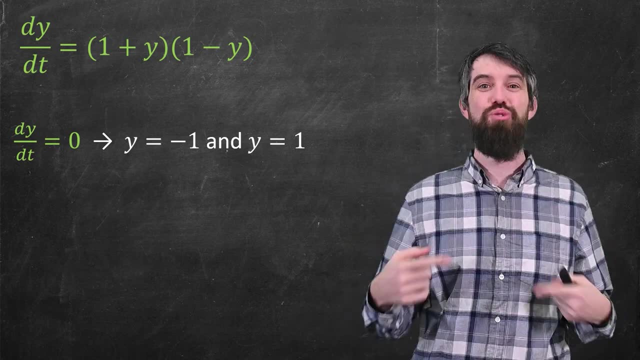 well, when is the derivative equal to 0, then you'd get that y is equal to minus 1 and y is equal to 1.. If you knew this was your derivative and you were in math 100, you'd say its critical. 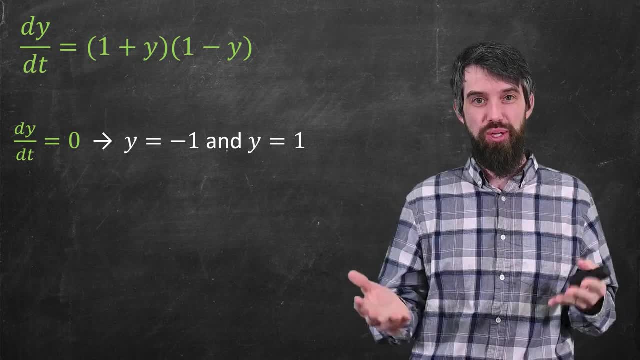 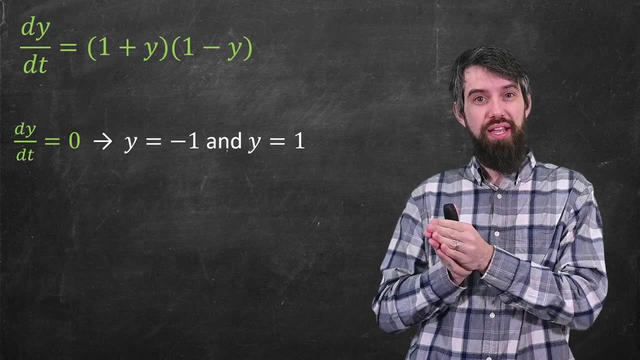 points were at minus 1 and 1, where the derivative was equal to 0.. So now we're going to turn to the computer to help us graph it, and I want you to keep these two spots- y equal to minus 1 and y equal to 1, in mind. So I'll open up my Jojoba to plot slope fields. 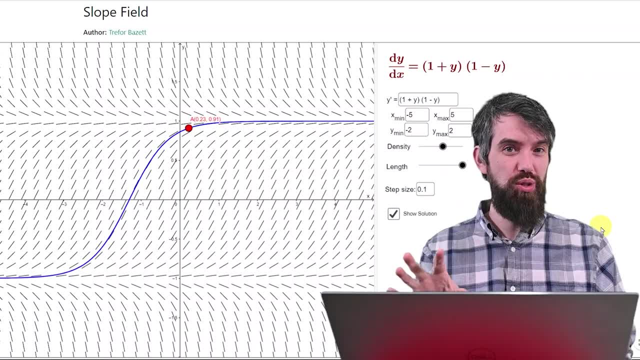 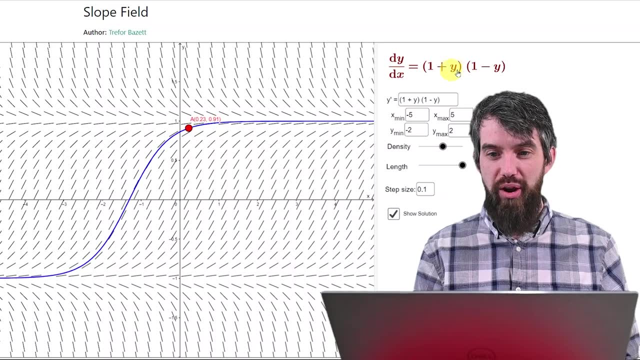 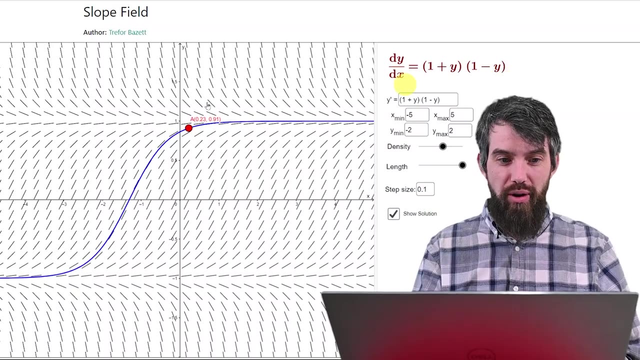 and I plugged in 1 plus y. 1 minus y is equal to y prime, And this is the kind of behavior that I get. So I want to notice a few things. First of all, recall that our two spots where the right-hand side was 0 was either y equal to 1 or y equal to minus 1.. And what you'll? 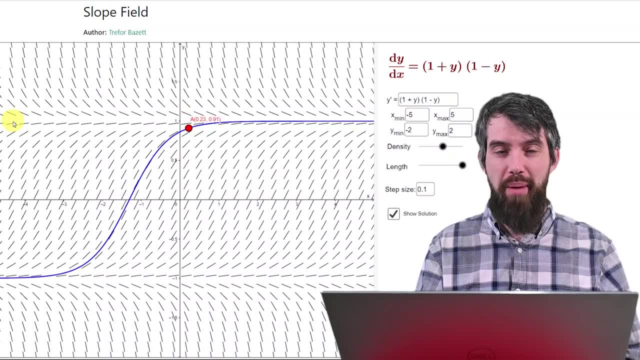 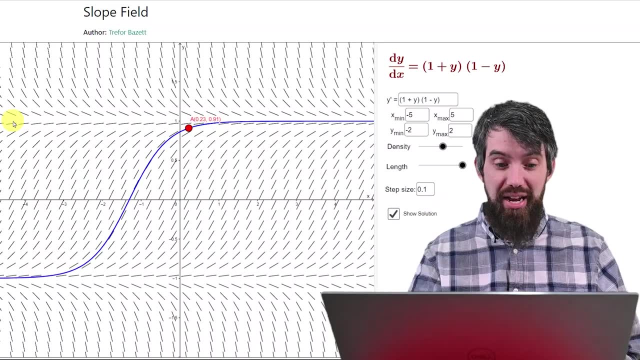 notice is if you go along the line y equal to 1 up here, it's where the derivative is 0. And if it plotted at that exact point you'd get horizontal lines, y is equal to minus 1.. That's down here. 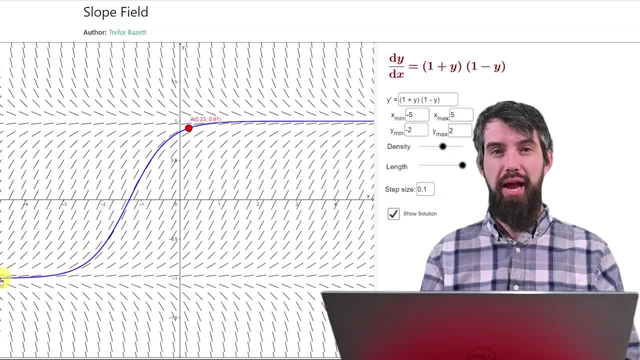 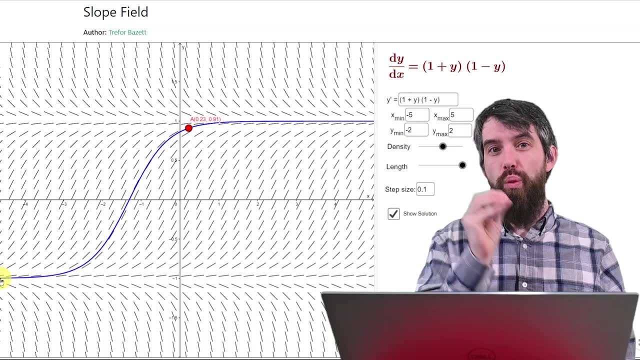 And minus 1, it's going to similarly be this horizontal line, And so these are what we call equilibrium solutions, And the idea of an equilibrium solution is: if you started at y equal to 1,, if your value is exactly y equal to 1, then the derivative would be: 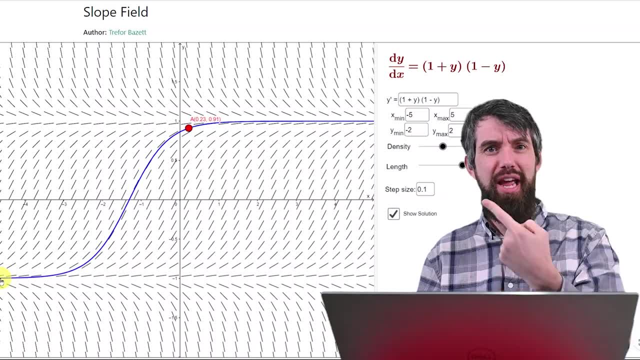 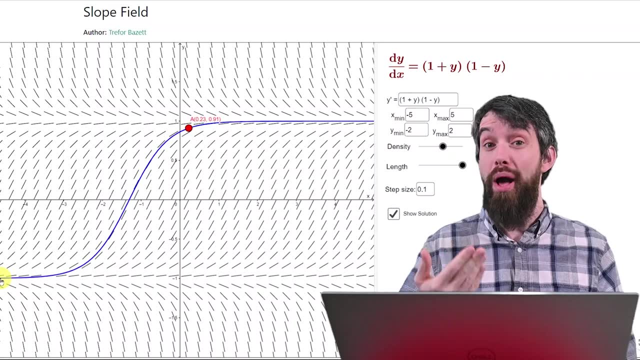 0, and so you wouldn't change, And then you wouldn't change, and then you wouldn't change. You'd always be at the value of y equal to 1.. That's why it's called an equilibrium position, because it doesn't change, And likewise for y equal to minus 1.. If you start at either 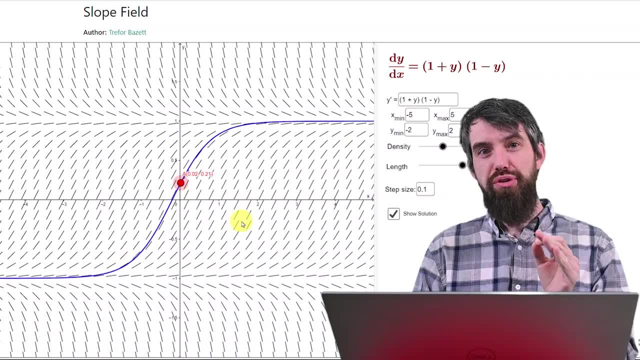 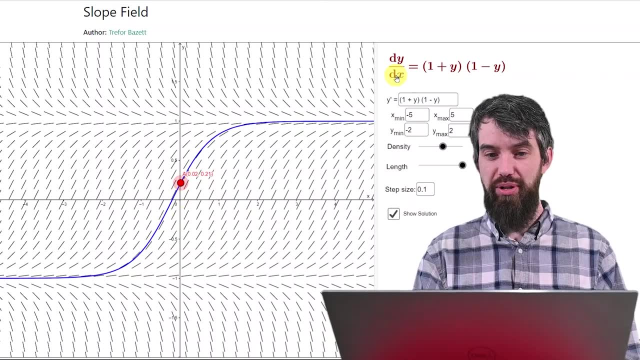 of those locations, then you just don't change at all. And the next thing I want you to notice is that, while this is a two-dimensional plot, so y is our vertical and our independent variable, which is labeled here as x, is our. 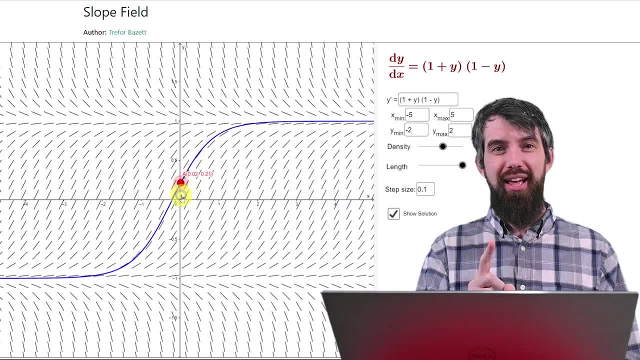 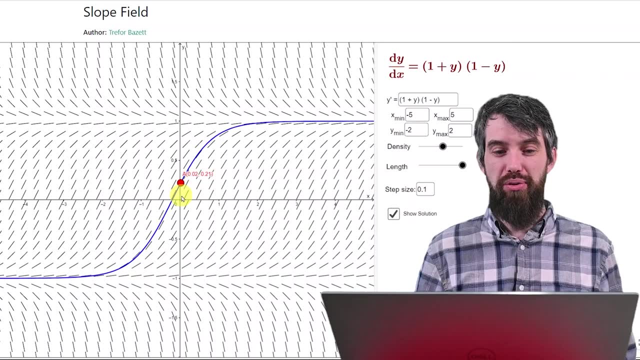 horizontal. while that is a two-dimensional plot, it's sort of only actually one-dimensional because the x doesn't matter. As in, everything is exactly the same along any horizontal line, Like take y equal to 0,, for example. If I was to plug in y equal to 0, I'd get a slope. 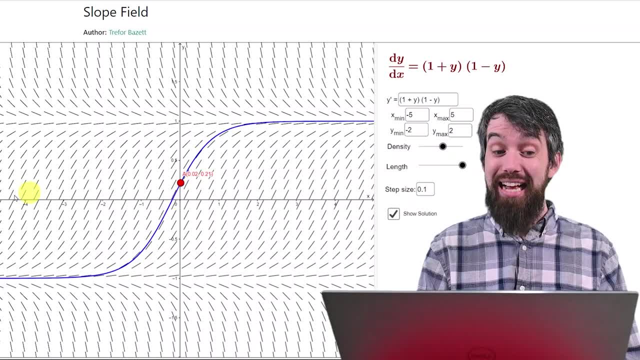 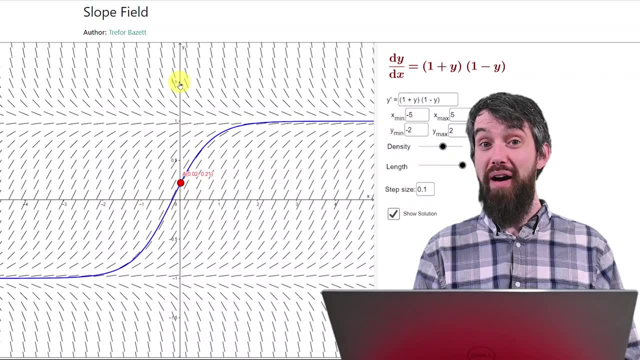 of 1.. All the way along the line, the x-axis, which is where y is equal to 0, the slope is exactly 1 there. And if you go to any point, okay, how about 1.5?? Well, 1.5 has. 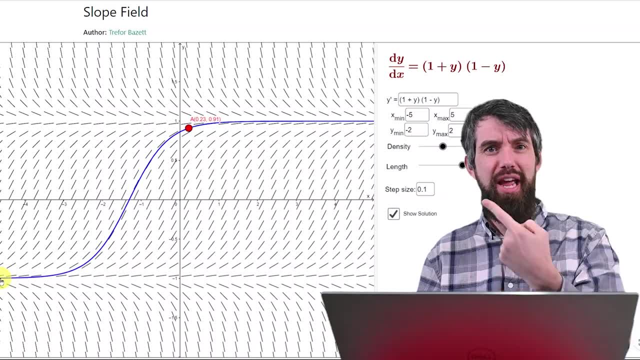 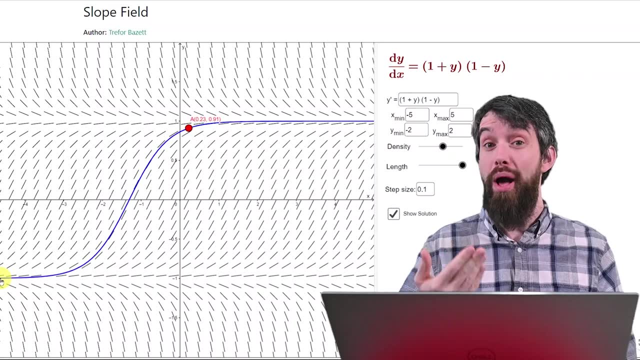 0, and so you wouldn't change, And then you wouldn't change, and then you wouldn't change. You'd always be at the value of y equal to 1.. That's why it's called an equilibrium position, because it doesn't change, And likewise for y equal to minus 1.. If you start at either 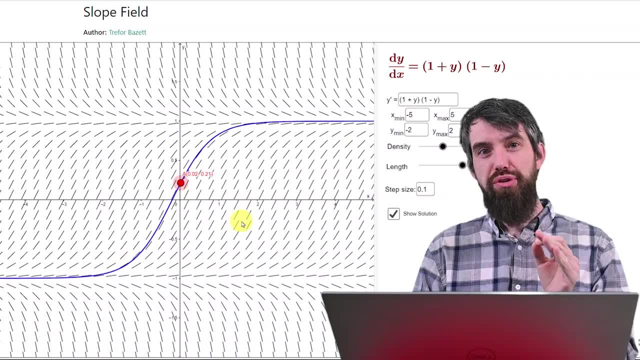 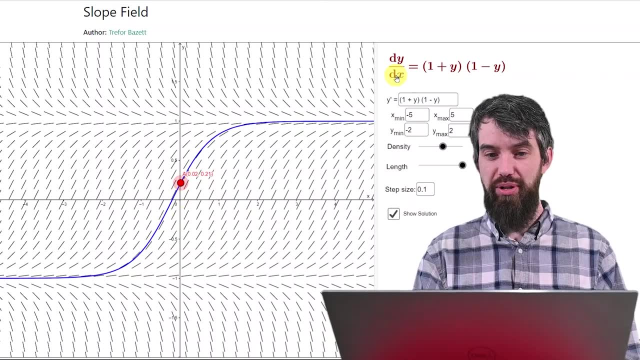 of those locations, then you just don't change at all. And the next thing I want you to notice is that, while this is a two-dimensional plot, so y is our vertical and our independent variable, which is labeled here as x, is our. 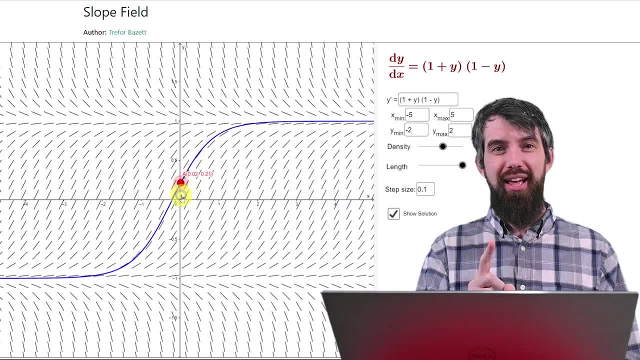 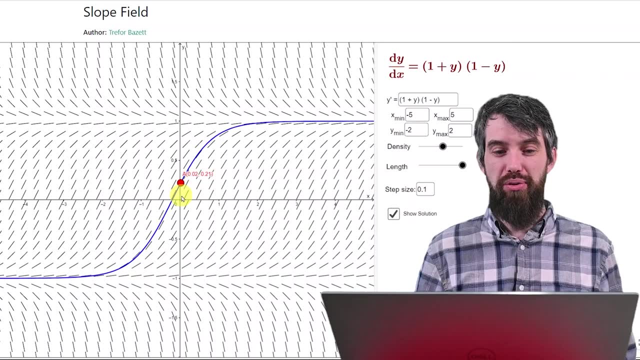 horizontal. while that is a two-dimensional plot, it's sort of only actually one-dimensional because the x doesn't matter. As in, everything is exactly the same along any horizontal line, Like take y equal to 0,, for example. If I was to plug in y equal to 0, I'd get a slope. 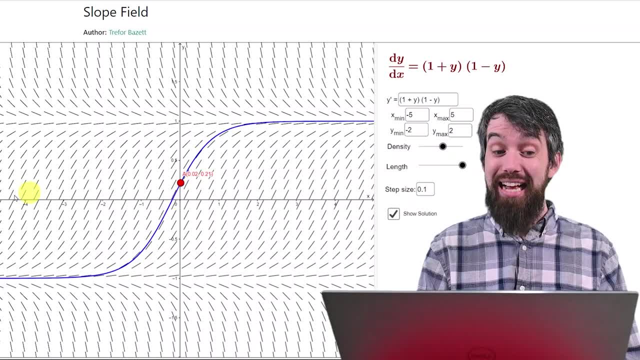 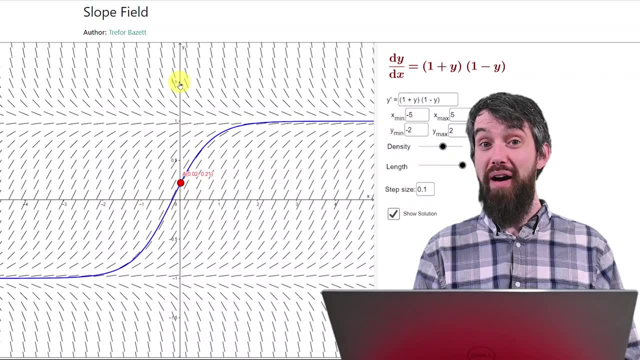 of 1.. All the way along the line, the x-axis, which is where y is equal to 0, the slope is exactly 1 there. And if you go to any point, okay, how about 1.5?? Well, 1.5 has. 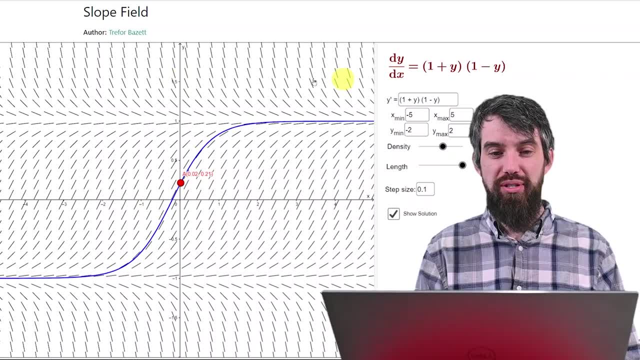 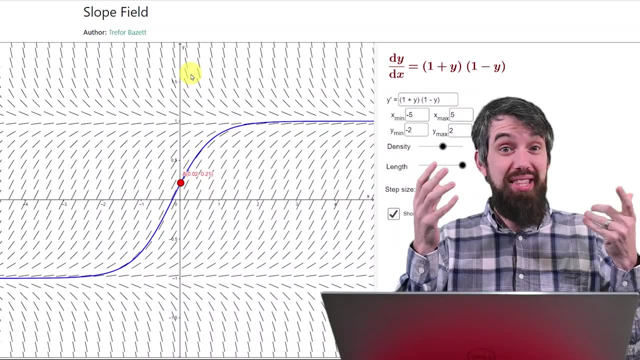 a steep negative slope. But if you go along the values of x, if you fix the value of y and just change x, it's the same slope everywhere. So, yes, it's a two-dimensional plot, but honestly, the information along the y-axis is really all that matters, because it's just the same. 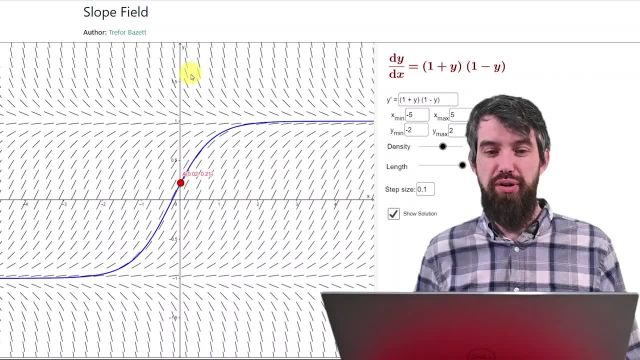 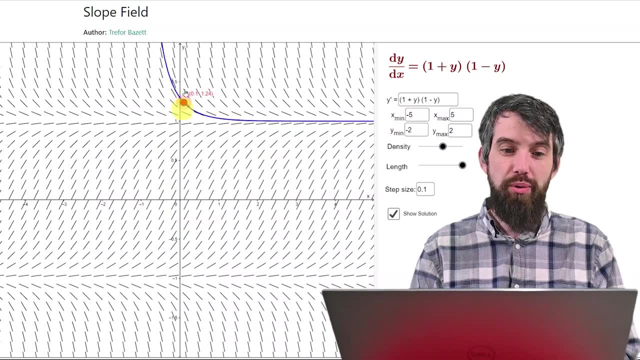 for every other value of x. All right. Third thing I want you to notice: I can take this starting initial condition and I can move around where it starts. I may as well just go up and down the y-axis to be talking about. x is equal to 0, what? 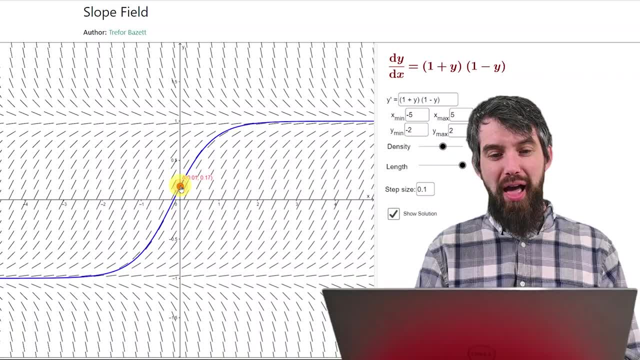 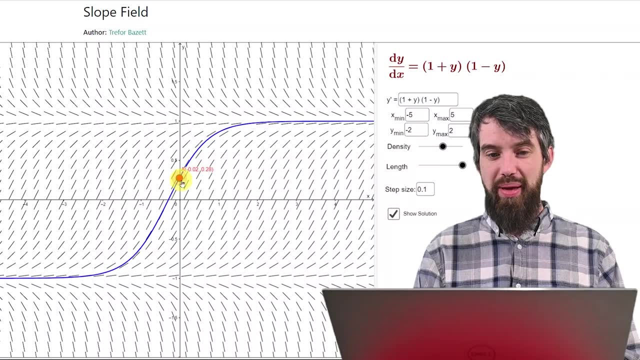 is the initial value of y, And if I'm in this region here, where I'm in between the two equilibrium values, then all of the curves look the same, Basically, if you increase the value of the independent variable, you go up to the one equilibrium. If you decrease it, you go down. 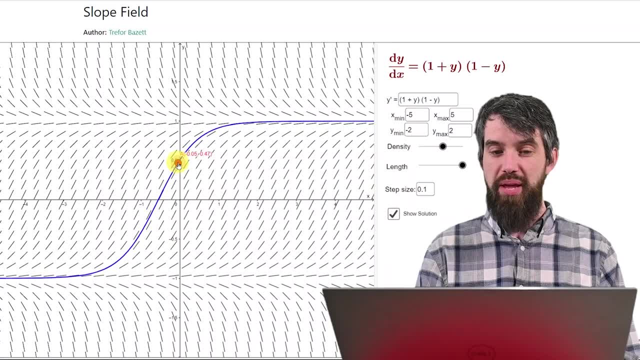 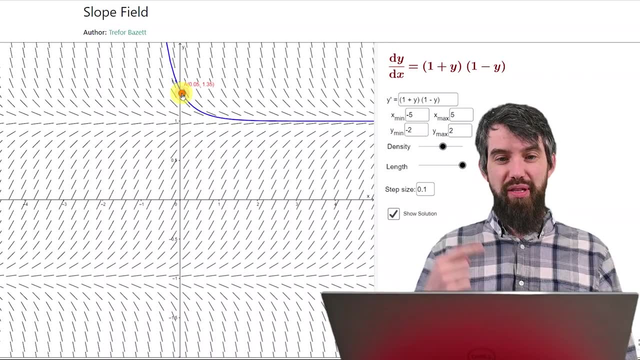 to the other equilibrium point, So they all have that basic shape. when I'm in between these two equilibrium points, If I was to go up above the equilibrium point so that now I was bigger than the value of 1, you'll notice that all of these curves 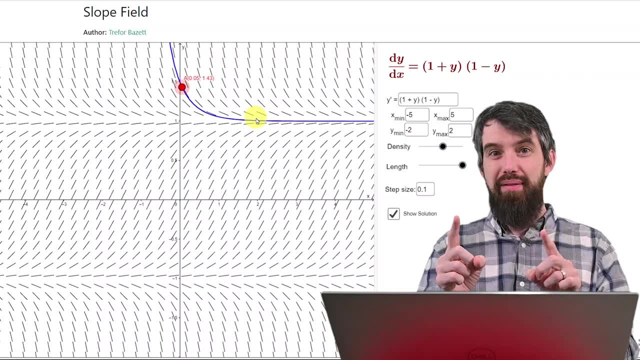 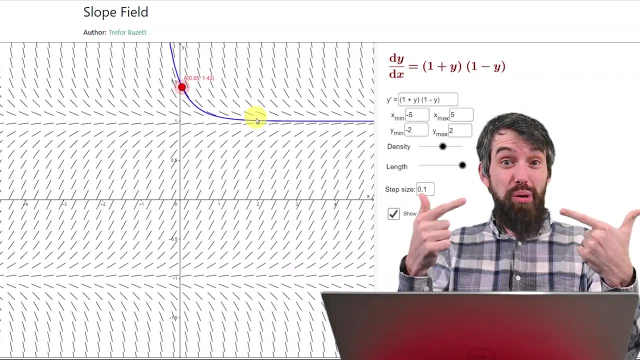 tend down towards the equilibrium point, but they don't cross it. So that's the big lesson here- is that when you've got these equilibrium points, you can't have a curve that crosses the equilibrium, because, well, if it ever hits the equilibrium, it just stays at the 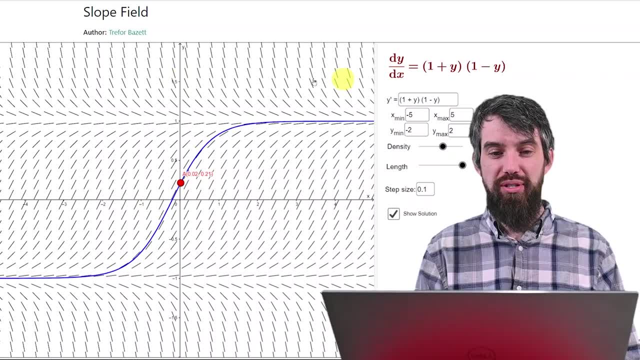 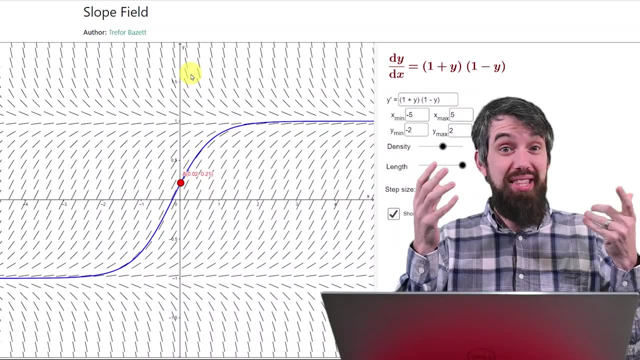 a steep negative slope. But if you go along the values of x, if you fix the value of y and just change x, it's the same slope everywhere. So, yes, it's a two-dimensional plot, but honestly, the information along the y-axis is really all that matters, because it's just the same. 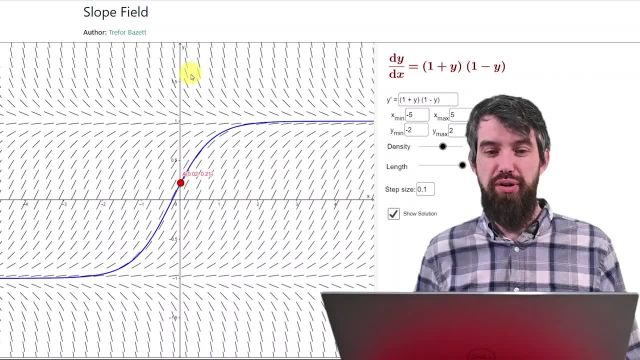 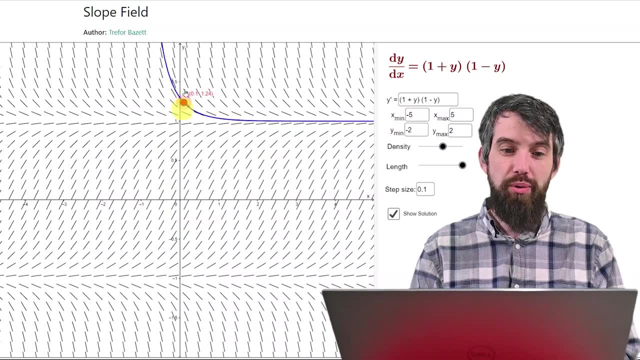 for every other value of x. All right. Third thing I want you to notice: I can take this starting initial condition and I can move around where it starts. I may as well just go up and down the y-axis to be talking about. x is equal to 0, what? 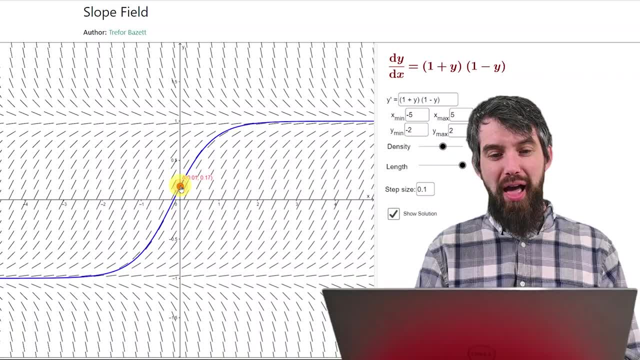 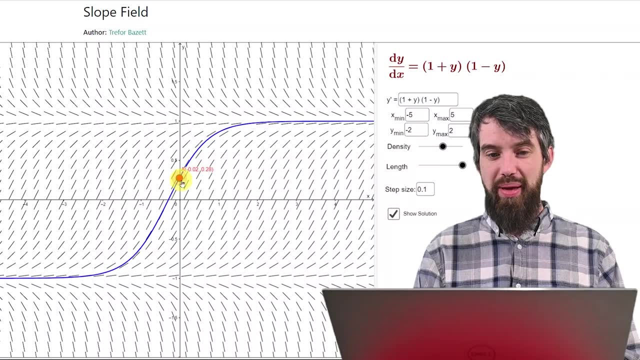 is the initial value of y, And if I'm in this region here, where I'm in between the two equilibrium values, then all of the curves look the same, Basically, if you increase the value of the independent variable, you go up to the one equilibrium. If you decrease it, you go down. 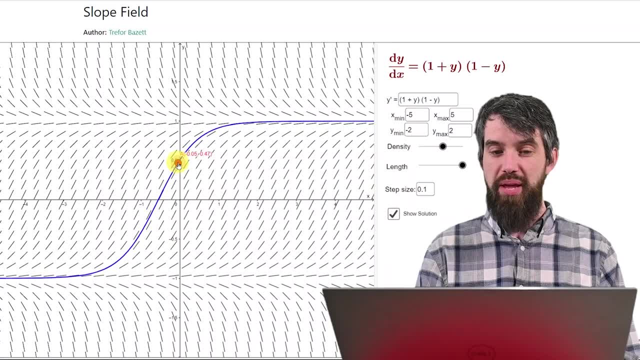 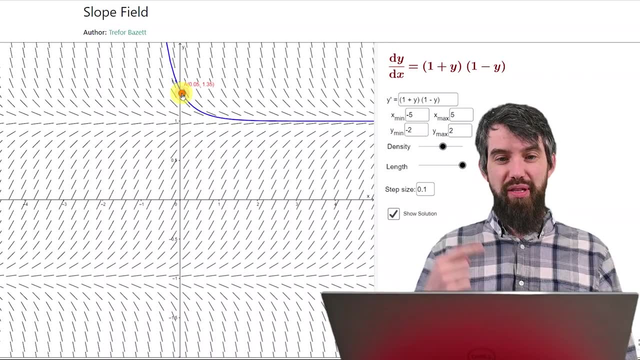 to the other equilibrium point, So they all have that basic shape. when I'm in between these two equilibrium points, If I was to go up above the equilibrium point so that now I was bigger than the value of 1, you'll notice that all of these curves 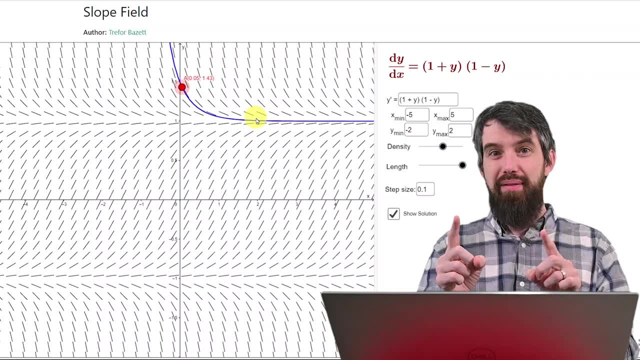 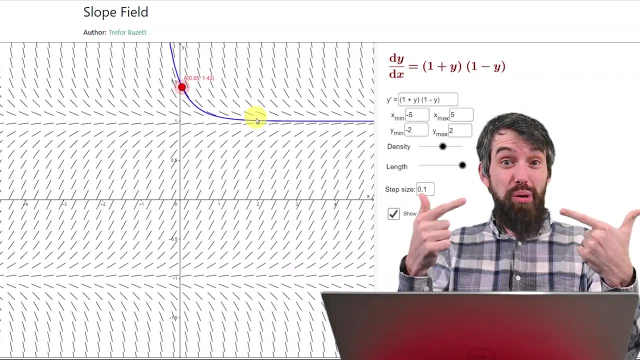 tend down towards the equilibrium point, but they don't cross it. So that's the big lesson here- is that when you've got these equilibrium points, you can't have a curve that crosses the equilibrium, because, well, if it ever hits the equilibrium, it just stays at the 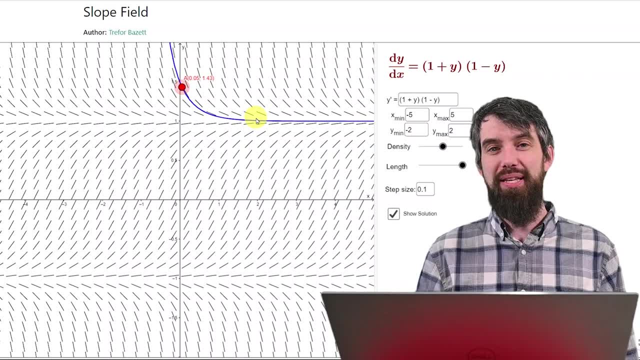 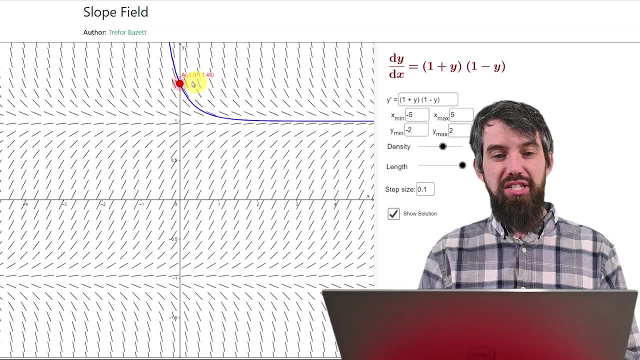 equilibrium forever. And then the final thing I want to note about this is that the two different equilibrium points have a very different type of behavior. Consider the y equal to 1 equilibrium point. If I start, as I've done here, above that equilibrium point, I'm going. 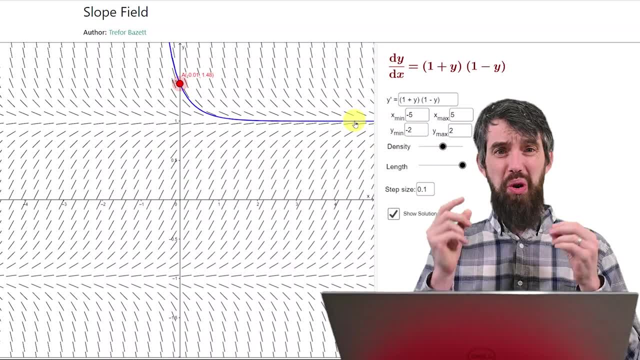 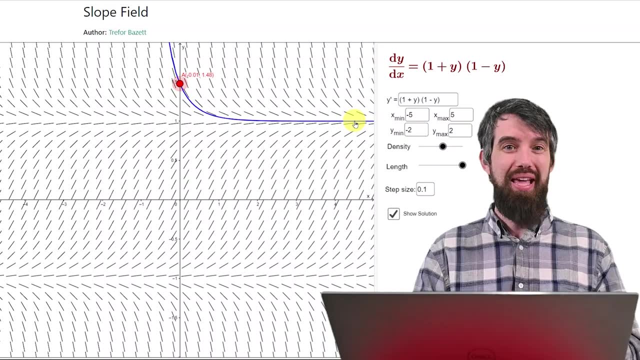 to descend until I basically end up really really near the equilibrium point. You can imagine that as time went to infinity you just sort of settled down right onto that equilibrium point. It would be asymptotically aligned with that equilibrium point And then 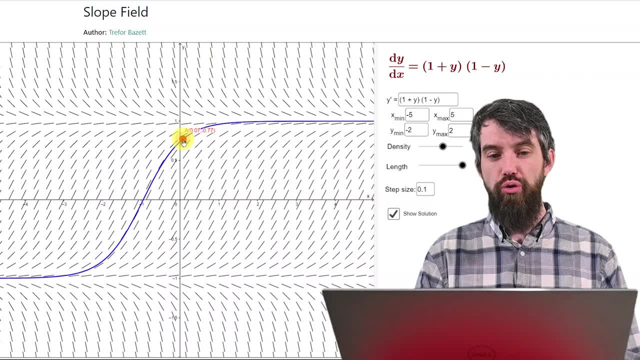 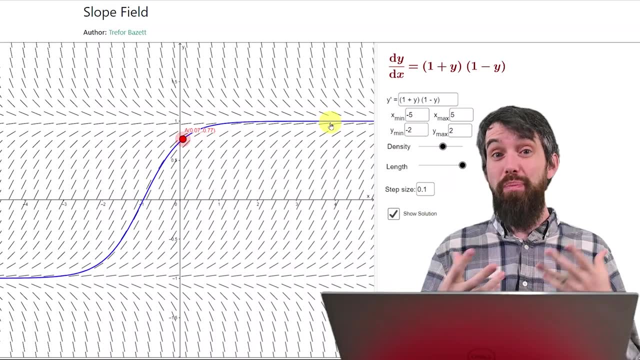 likewise, if you began a little bit beneath the equilibrium point, you rise up until you get to that equilibrium point. This is what we're going to call asymptotically stable. It basically says: if you're nearby the equilibrium point, you're going to end up at that equilibrium. 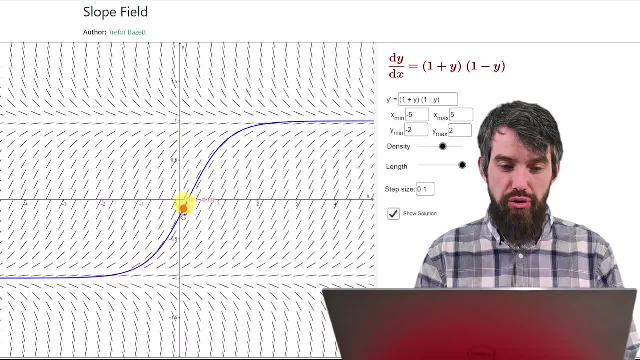 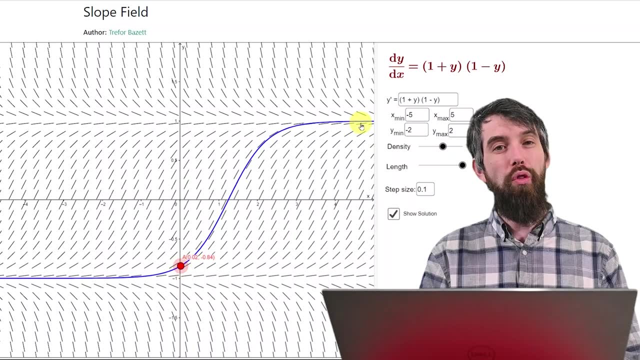 point. Let's contrast this with what happens if you start near the value of y equal to minus 1.. I mean, I'm right here, near the value of y equal to minus 1, but it sends you all the way up to plus 1 again. Likewise, if I start just beneath the value of minus 1,, okay, I'm. 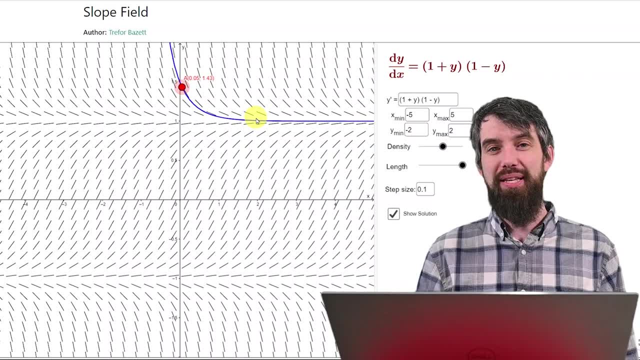 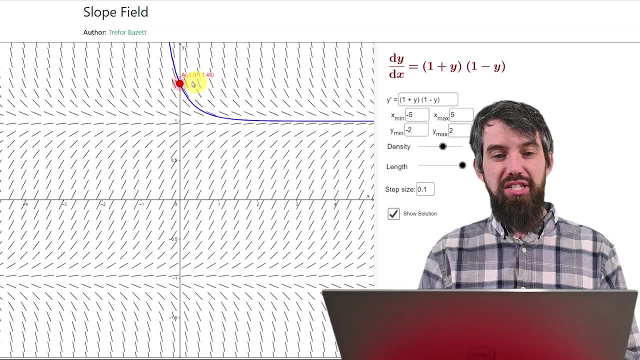 equilibrium forever. And then the final thing I want to note about this is that the two different equilibrium points have a very different type of behavior. Consider the y equal to 1 equilibrium point. If I start, as I've done here, above that equilibrium point, I'm going. 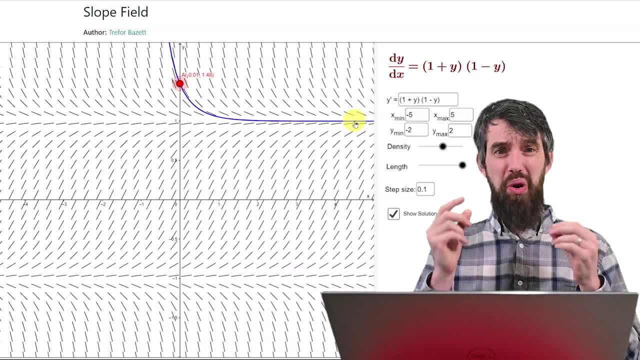 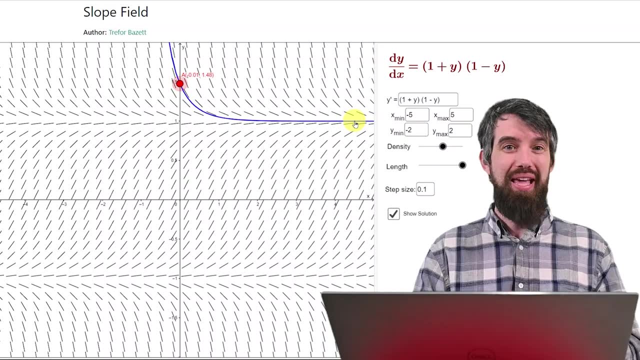 down to the equilibrium point. I descend until I basically end up really, really near the equilibrium point. You can imagine that as time went to infinity you just sort of settled down right onto that equilibrium point. It would be asymptotically aligned with that. 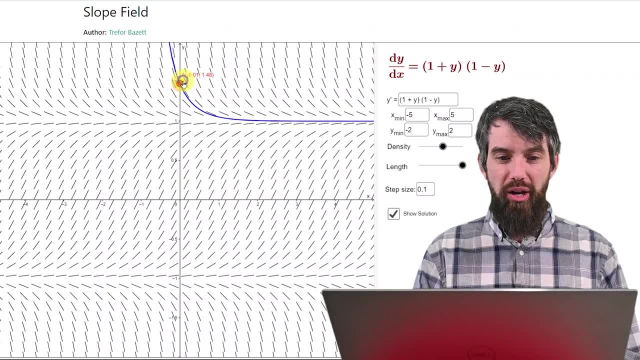 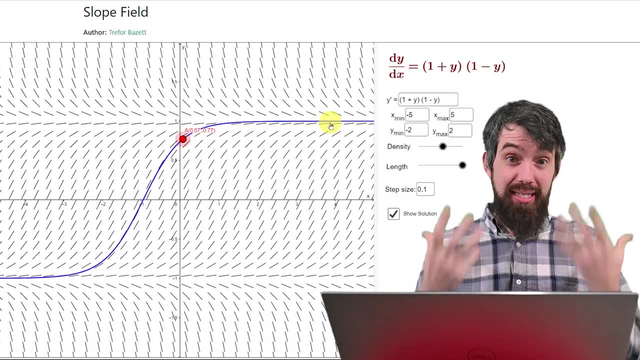 equilibrium point. And then, likewise, if you began a little bit beneath the equilibrium point, you rise up until you get to that equilibrium point. This is what we're going to call asymptotically stable. It basically says: if you're nearby the equilibrium point, you're going to end. 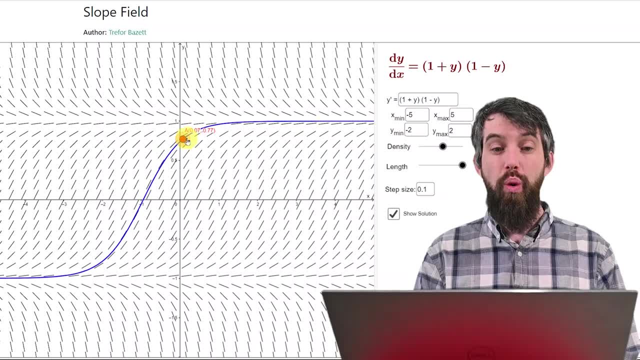 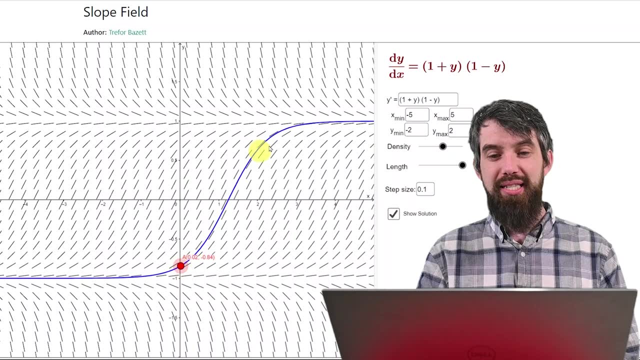 up at that equilibrium point. And then I'm going to contrast this with what happens if you start near the value of y equal to minus 1.. I mean, I'm right here, near the value of y equal to minus 1, but it sends. 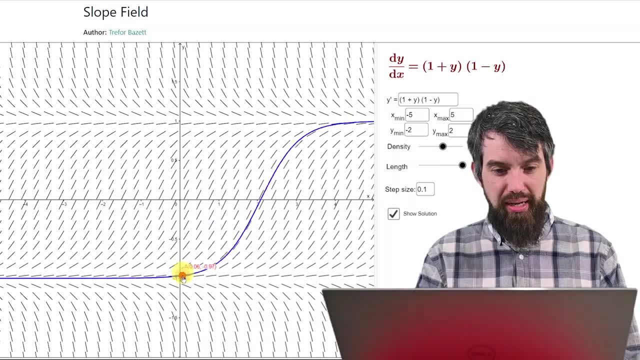 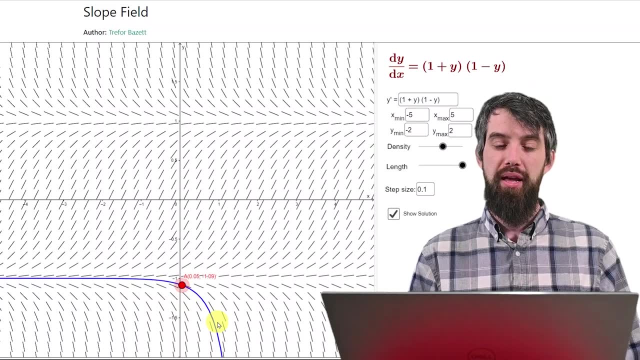 you all the way up to plus 1 again. Likewise, if I start just beneath the value of minus 1, OK, I'm very close to that equilibrium point, but it sends you away, looking like it's going to minus infinity. This type of equilibrium point where solutions that start. 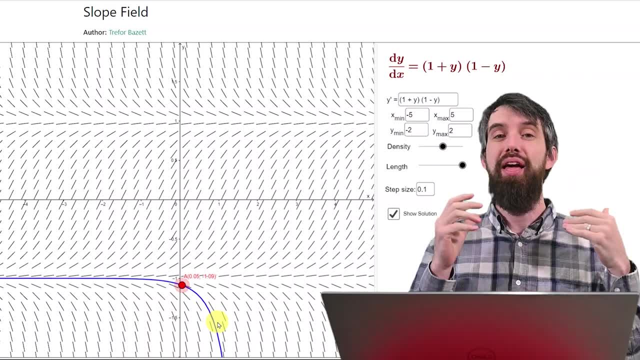 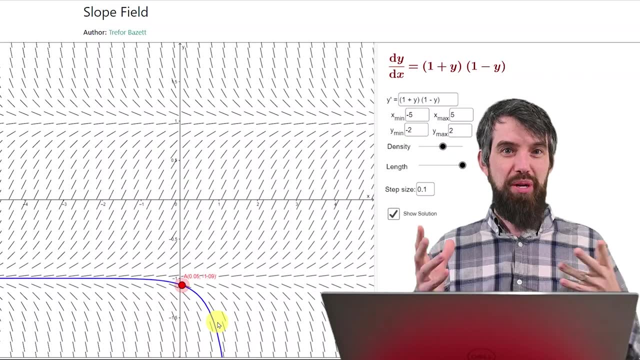 nearby tend to go off in completely different directions, is called an unstable equilibrium point. And then this is called an unstable equilibrium point. OK, so that's pictorially what's going on. Let's just write down these definitions a bit more precisely. 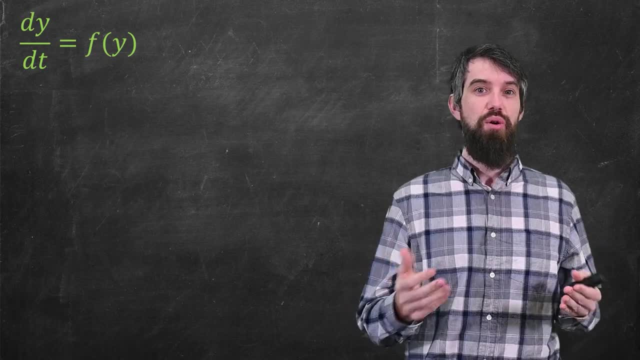 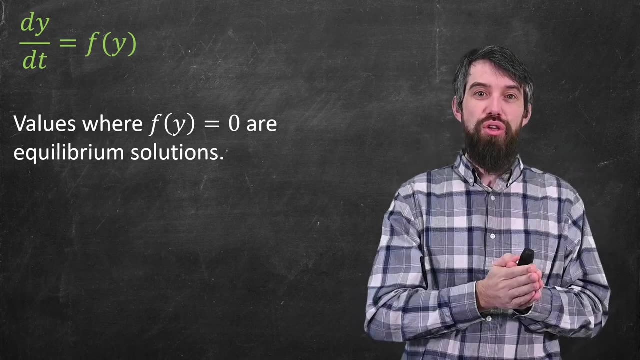 OK, so now let's write down those definitions Precisely. we have here a generic, autonomous equation. An equilibrium solution is a constant solution whose value is just a zero of the function f of y. It's a spot where f of y is equal to zero, And we're calling it an. 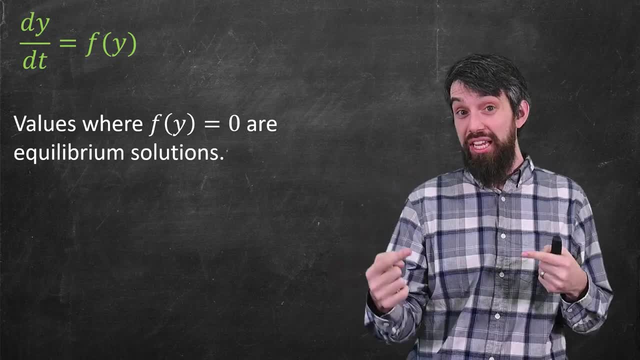 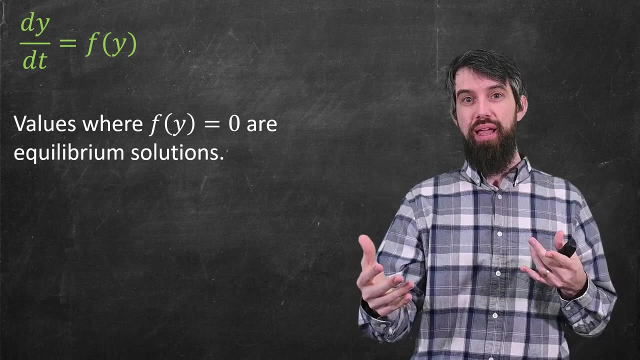 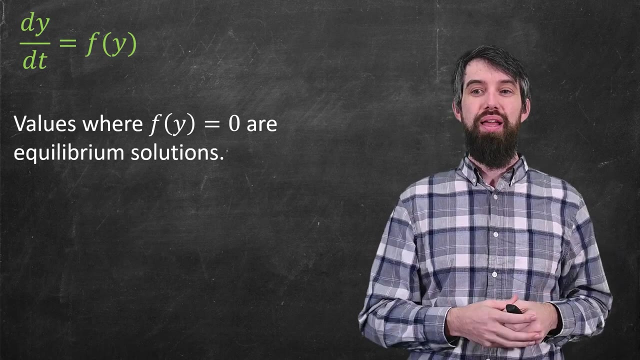 equilibrium solution, because the rate of change of y at that spot is zero And so nothing changes. It's just sort of static, Hence an equilibrium solution. And then what we saw is that there's actually a couple possibilities that equilibrium solutions can look different ways. One of them is they can be called asymptotically stable. And what? 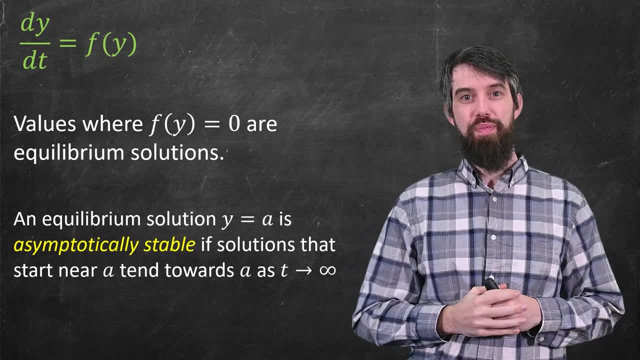 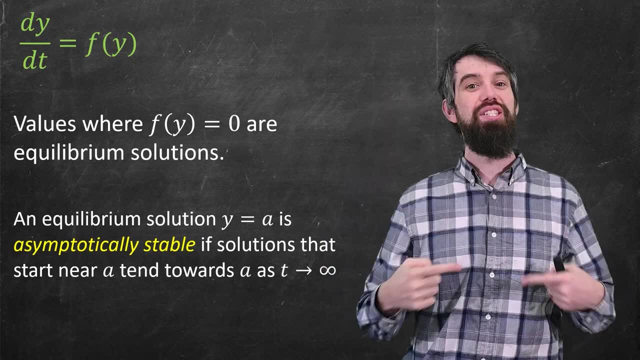 we meant by this is that if you had an equilibrium solution, y equal to a, and you started nearby a- maybe not exactly at a, but in some region around a- then as time went on, you're going to get closer and closer and closer to the value of a. You're going to tend to get closer. 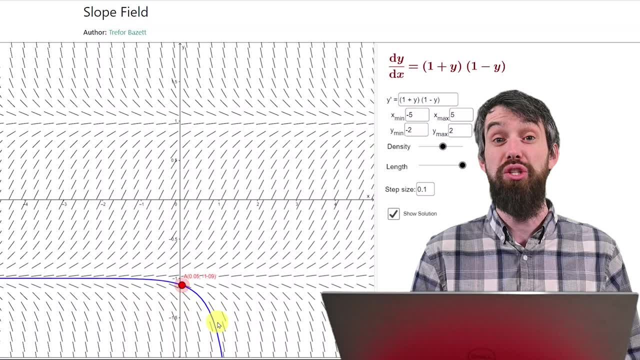 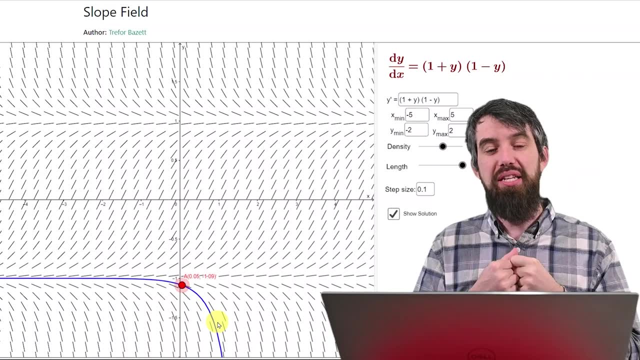 very close to that equilibrium point, but it sends you away looking like it's going to minus infinity. This type of equilibrium point, where solutions that start nearby tend to go off in completely different directions, is called an unstable equilibrium point, as opposed to a stable equilibrium point. 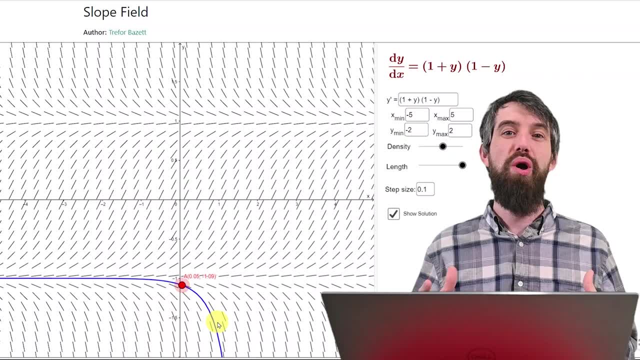 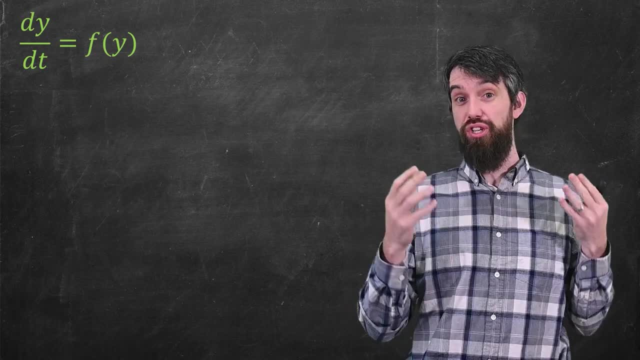 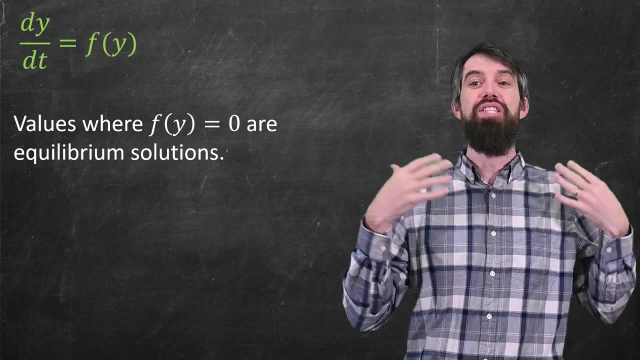 Okay, so that's pictorially what's going on. Let's just write down these definitions a bit more precisely. Okay, so now let's write down those definitions precisely. We have here a generic, autonomous equation. An equilibrium solution is a constant solution whose value is just a zero of the 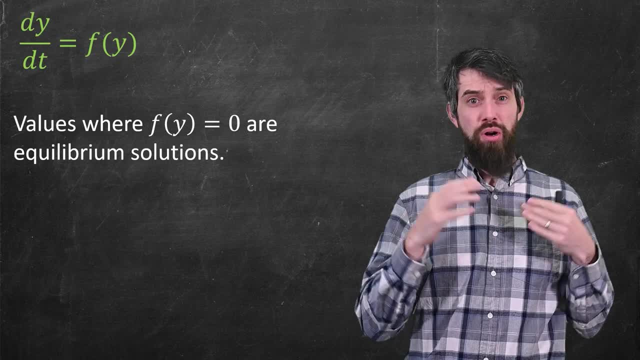 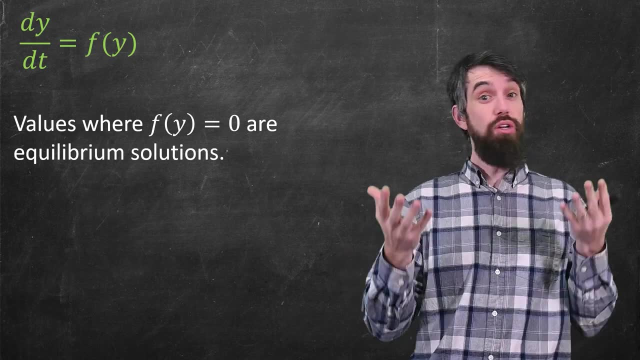 function f of y. It's a spot where f of y is equal to zero And we're calling it an equilibrium solution, because the rate of change of y at that spot is zero And so nothing changes. It's just sort of static and hence an equilibrium solution. And then what we 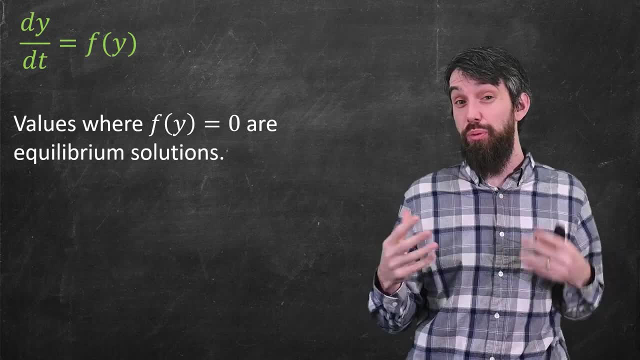 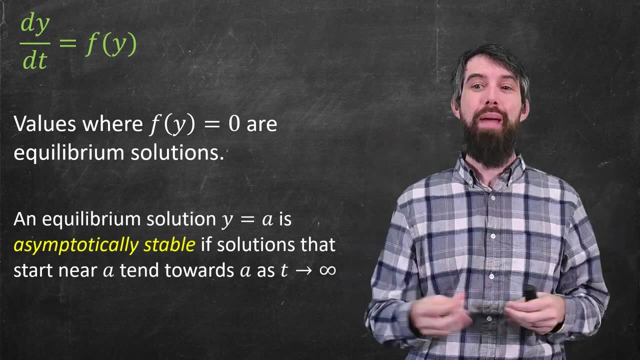 saw is that there's actually a couple possibilities that equilibrium solutions can look different ways. One of them is they can be called asymptotically stable, And what we meant by this is that if you had an equilibrium solution y equal to a and you started nearby, a maybe not. 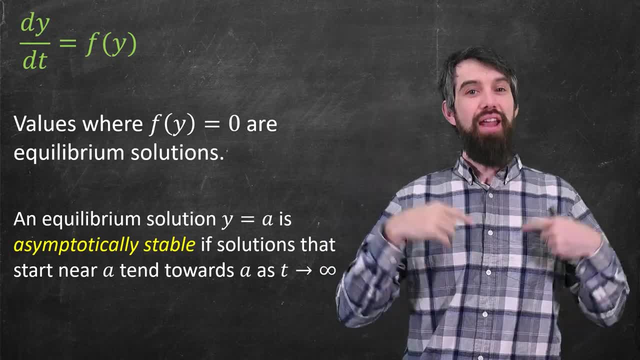 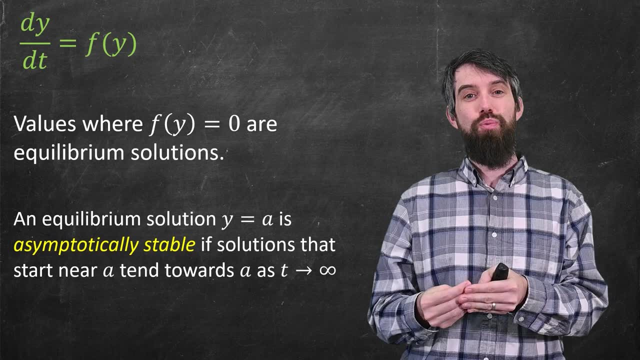 exactly at a, but in some region around a. then, as time went on, you're going to get closer and closer and closer to the value of a. You're going to tend towards the equilibrium. So this is when you have an asymptotically stable situation. It basically says: if you 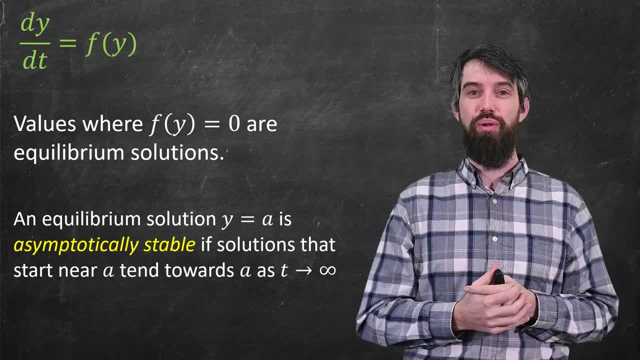 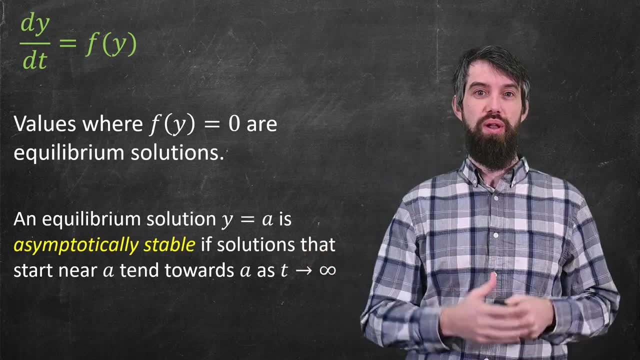 start nearby the equilibrium solution, you're going to end up at the equilibrium solution, at least if you had enough time, as time goes to infinity. This was in contrast to an unstable equilibrium point, And an unstable equilibrium value is the opposite. If you start near the 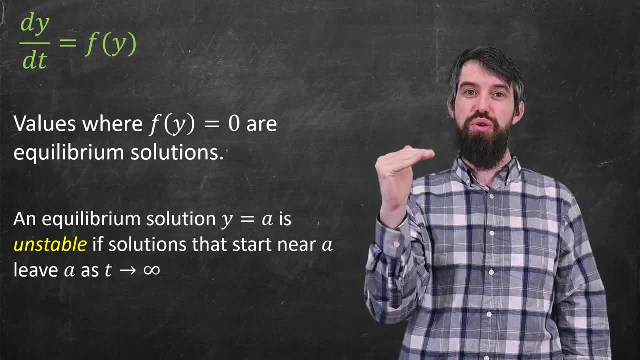 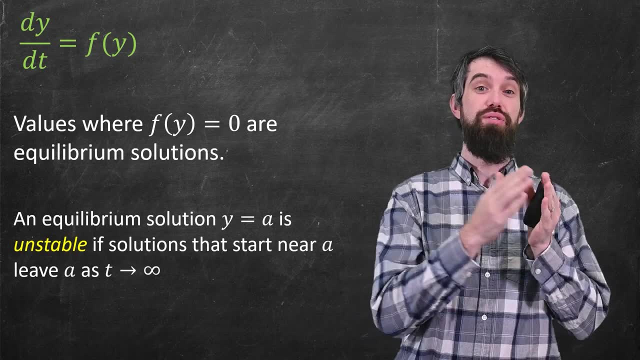 value of y equal to a. even if you start extremely close to the value of a, then you're going to leave the value of a as time goes on, And so equilibrium solutions are either stable or unstable. Now, the final thing I want to do is return to the equation that we've seen: the slope. 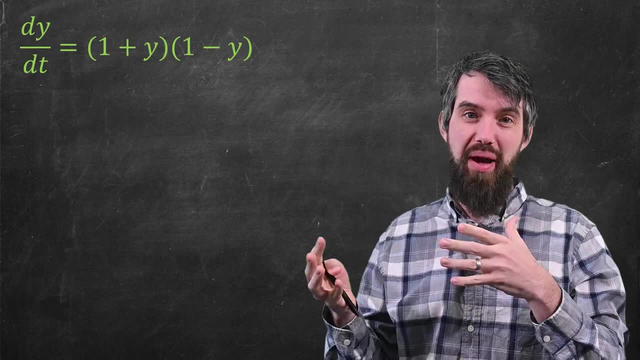 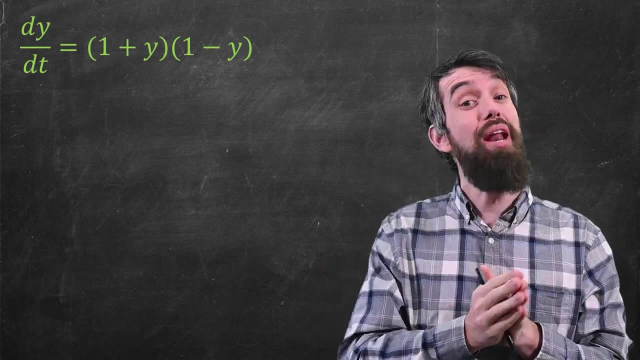 field before That's y prime is 1 plus y times 1 minus y. And to talk just a little bit more about the equilibrium solutions and whether they're stable or unstable- And this time I'm going to actually draw it out by hand as opposed to turning to the computer. It's: 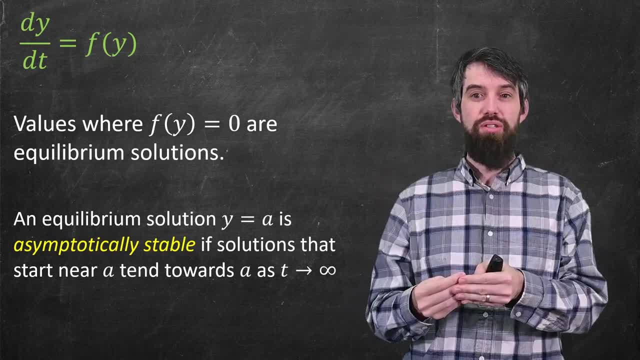 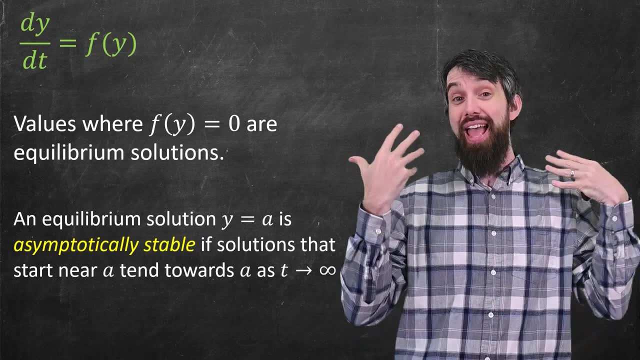 and closer to the value of a, You're going to tend to get closer and closer and closer, going to tend towards the value of a. So this is when you have an asymptotically stable situation. It basically says: if you start nearby the equilibrium solution, you're going to end up at 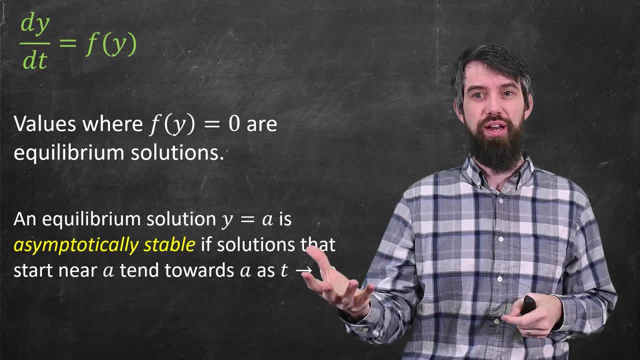 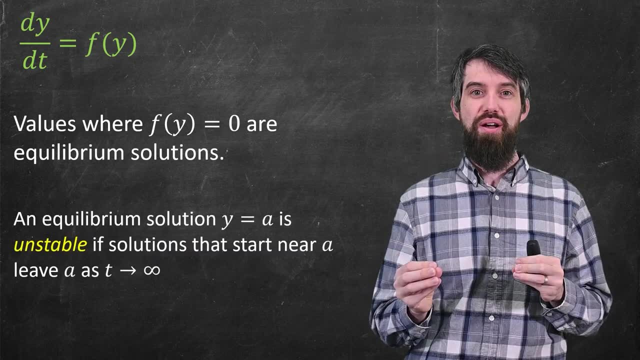 the equilibrium solution, at least if you had enough time, as time goes to infinity. This was in contrast to an unstable equilibrium point, And an unstable equilibrium value is the opposite. If you start near the value of y equal to a, even if you start extremely close to the value of a, 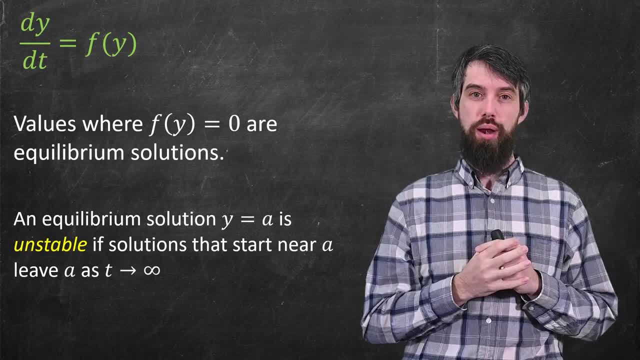 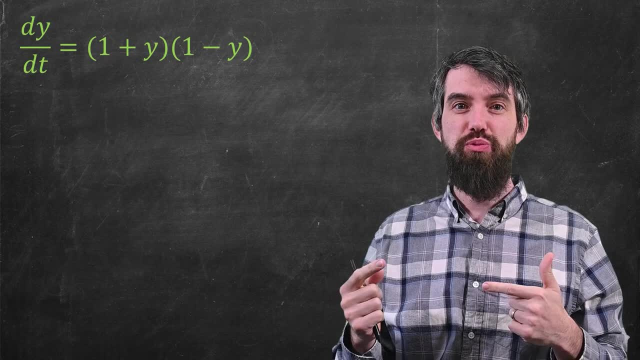 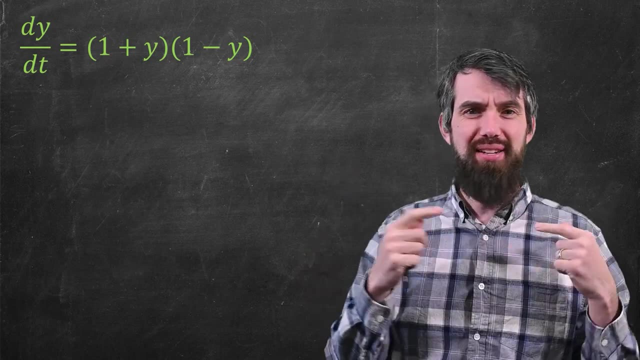 then you're going to leave the value of a as time goes on, And so equilibrium solutions are either stable or unstable. Now the final thing I want to do is return to the equation that we've seen, the slope field before, that's, y prime is 1 plus y times 1 minus y, and to talk just a little bit, 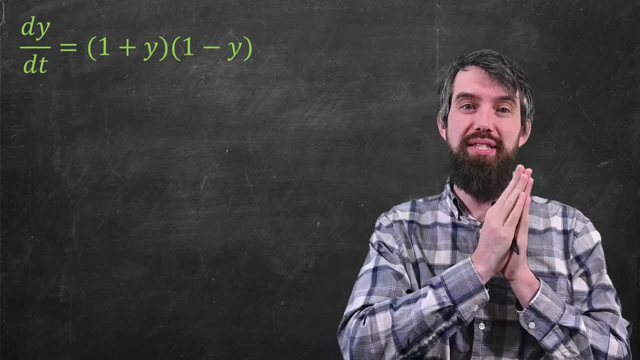 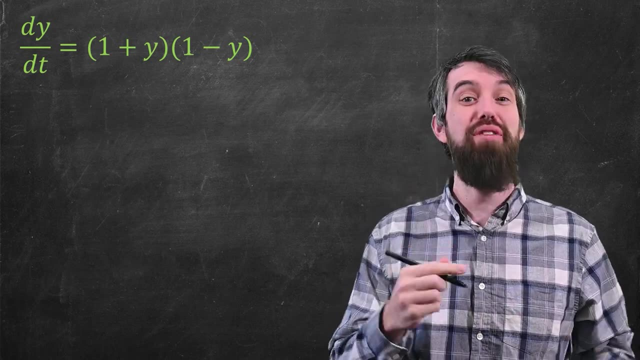 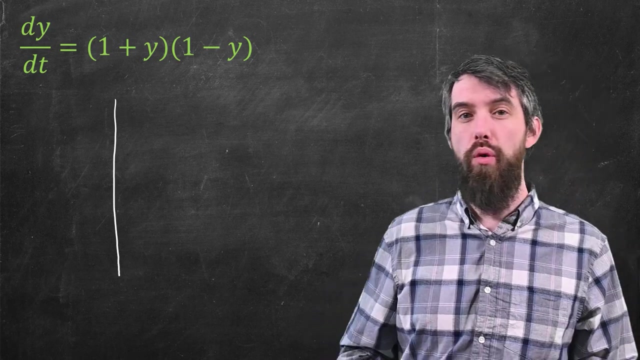 more about the equilibrium solutions and whether they're stable or unstable. And this time I'm going to actually draw it out by hand as opposed to turning to the computer. It's actually not so bad when you have an autonomous equation, Because recall that this only depends on y, So I don't really need to do anything more than draw the y-axis. 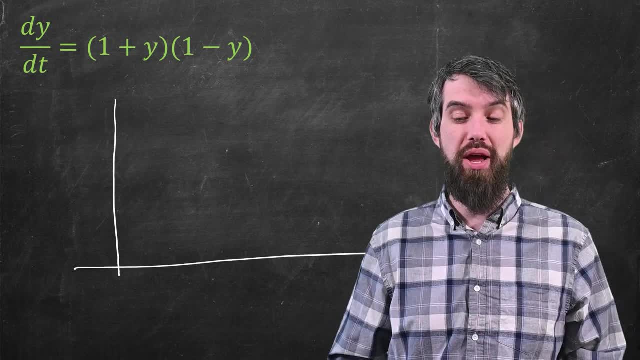 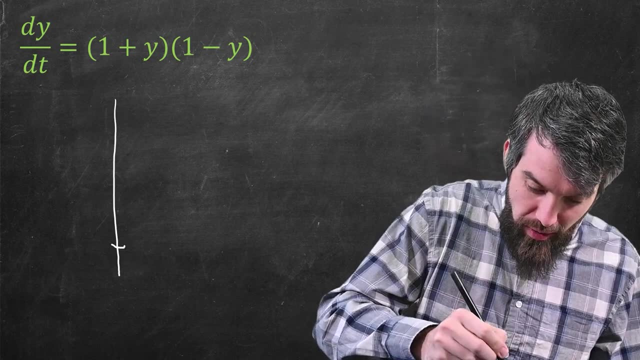 I could draw the t-axis, that would be going off to the right, but why? It's the same for all values of t, so let me ignore this. And then the next thing I'd like to do is I'd like to come here and put on the equilibrium value. 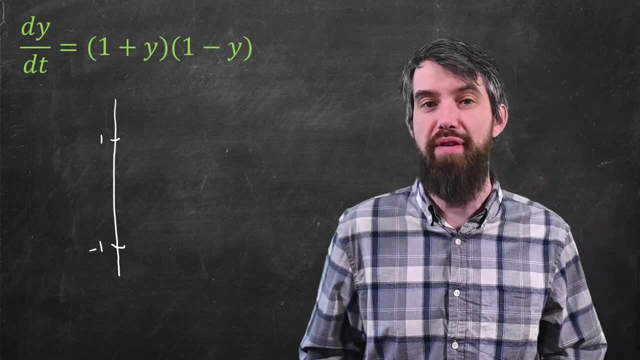 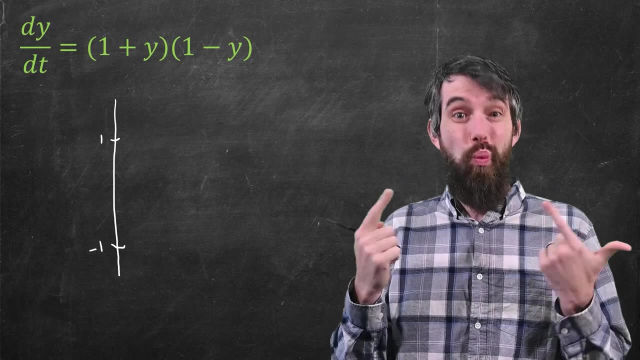 So I have the minus 1 and the 1.. Those were the two different equilibrium values that I found, And then what I'd really like to do is to look above and below every one of these equilibrium values and just say: what is the slope doing at that point? 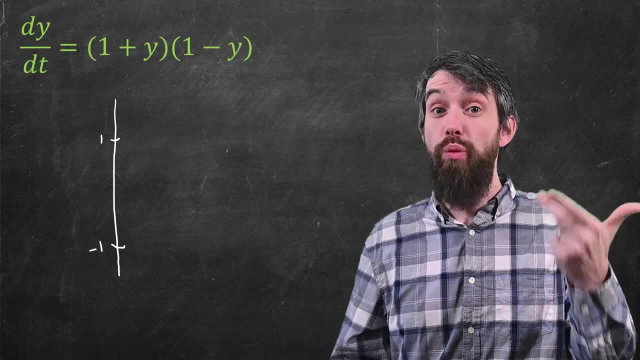 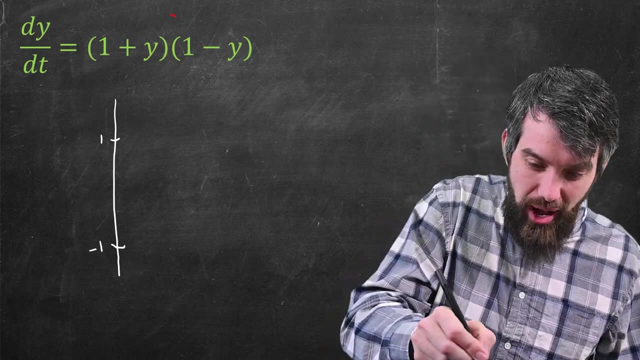 So let me start by looking at values bigger than 1, bigger than the larger of the two equilibrium points, For example 2 as just a number, If I was to come in here and to plug in the value of 2 there and the value of 2 there. 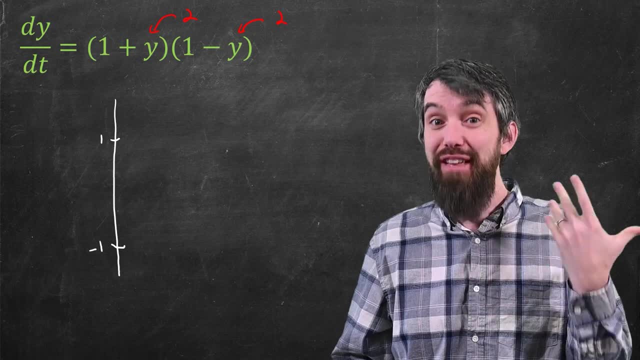 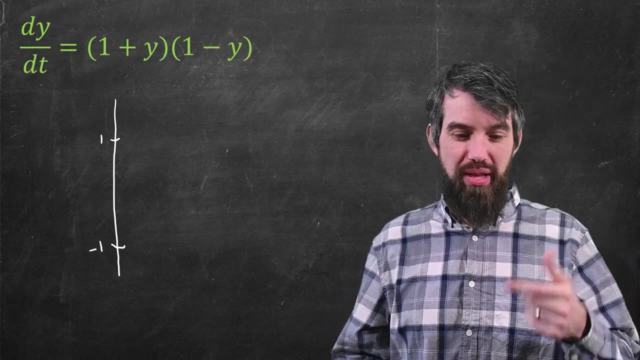 then what I would get was a negative number. Indeed, any value bigger than 1 is going to give me a negative, because this right term is going to dominate and be negative, And the way I'm going to illustrate this is to go and draw a. 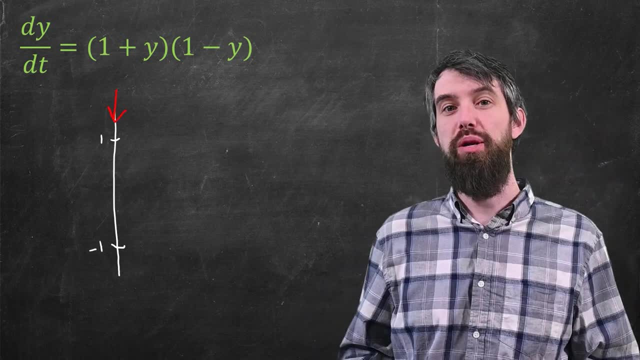 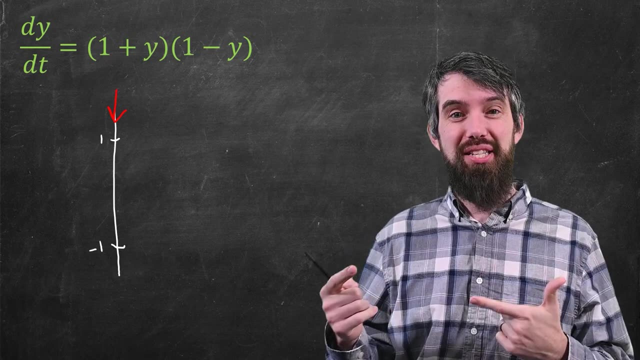 downward arrow when I'm above that first equilibrium point. So this is just indicating that my slope is negative, that it's going to be going down, that the values of y will be dropping. This is very reminiscent of what we did back in Calculus 1 when we were studying the critical points of a function. 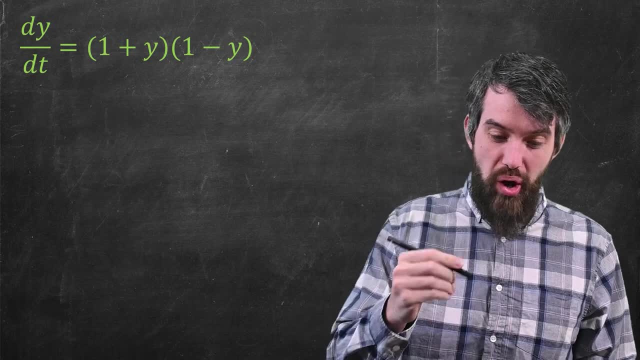 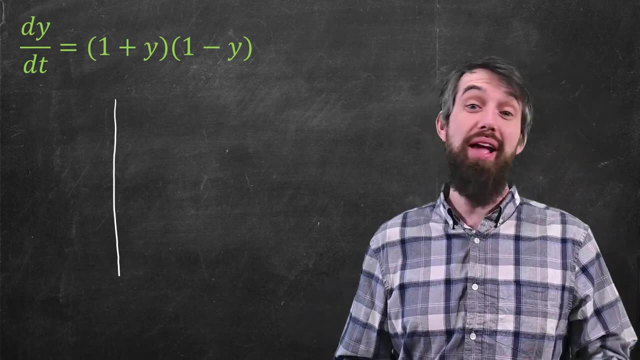 actually not so bad when you have an autonomous equation, because recall that this only depends on y, So I don't really need to do anything more than draw the y-axis. I could draw the t-axis, that would be going off to the right. 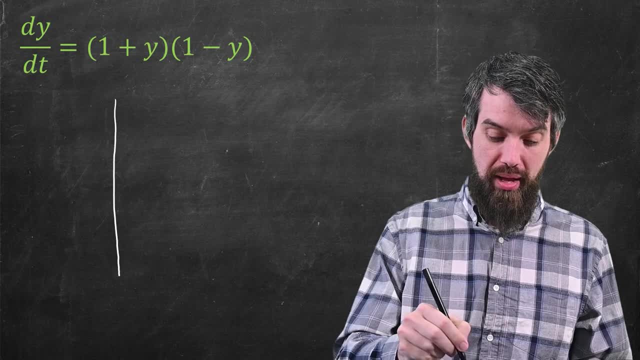 but why It's the same for all values of t. so let me ignore this. And then the next thing I'd like to do is I'd like to come here and put on the equilibrium value. So I have the minus one and the one. 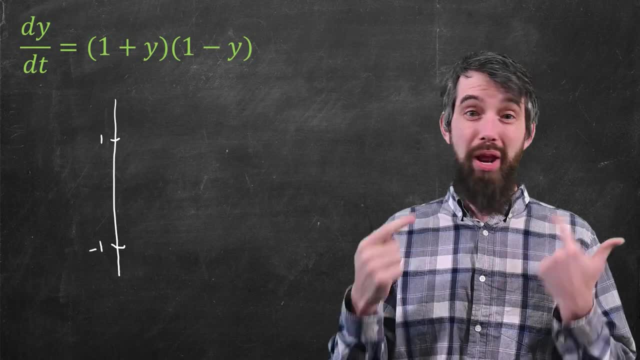 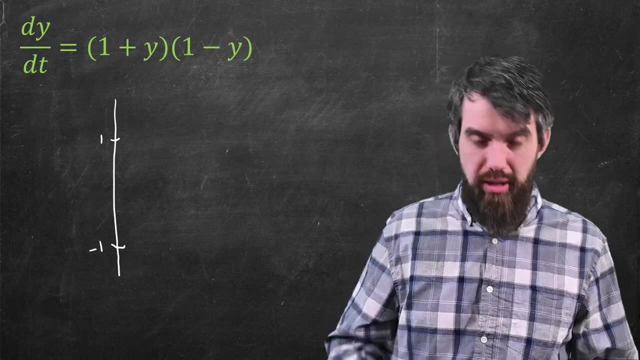 Those were the two different equilibrium values that I found, And then what I'd really like to do is to look above and below every one of these equilibrium values and just say: what is the slope doing at that point? So let me start by looking at values bigger than one. 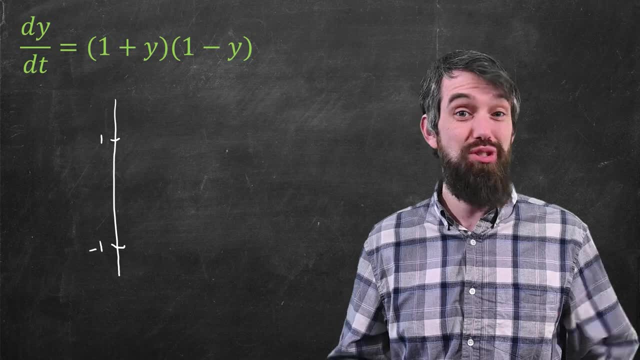 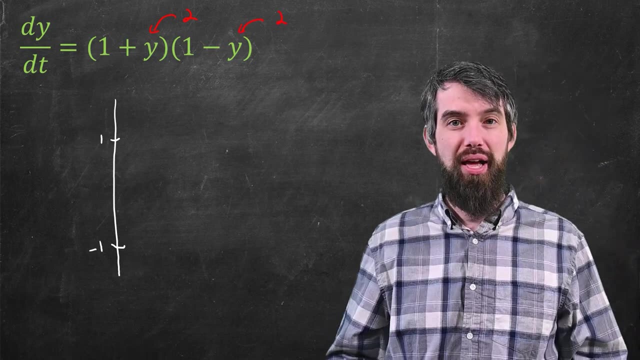 bigger than the larger of the two equilibrium points. For example, two as just a number. If I was to come in here and to plug in the value of two there and the value of two there, then what I would get was a negative number. 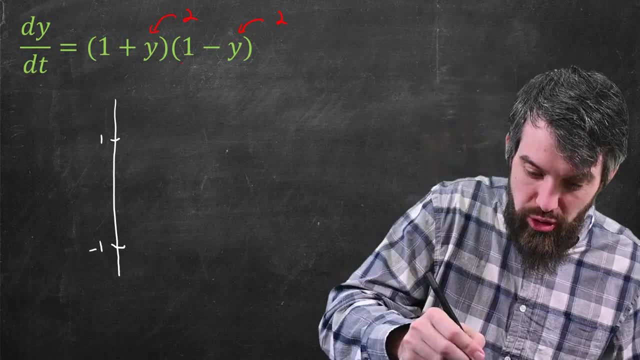 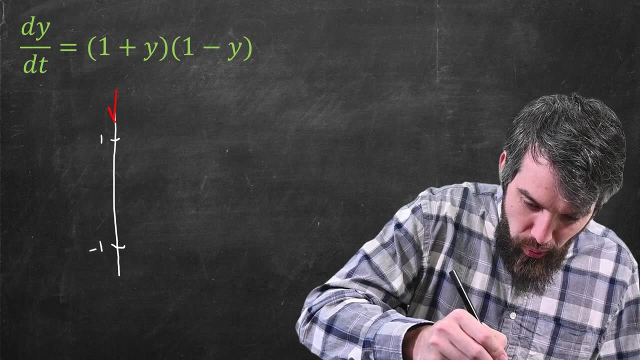 And indeed any value bigger than one is gonna give me a negative, because this right term is gonna dominate and be negative, And the way I'm gonna illustrate this is to go and draw a downward arrow when I'm above that first equilibrium point. So this is just indicating that my slope is negative. 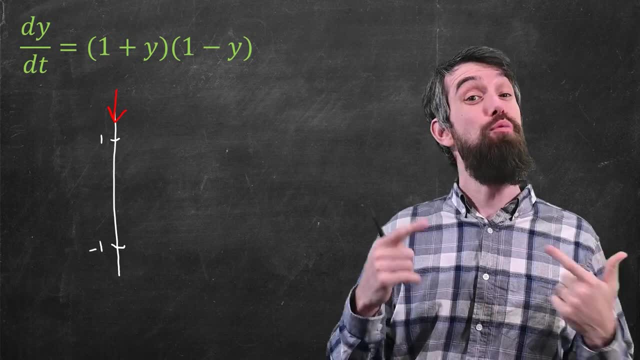 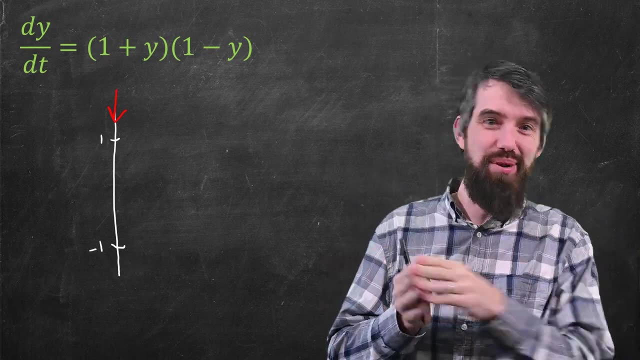 that it's gonna be going down, that the values of y will be dropping. This is very reminiscent of what we did back in calculus one, when we were studying the critical points of a function and we looked to the left and the right and see whether the derivative was positive or increased. 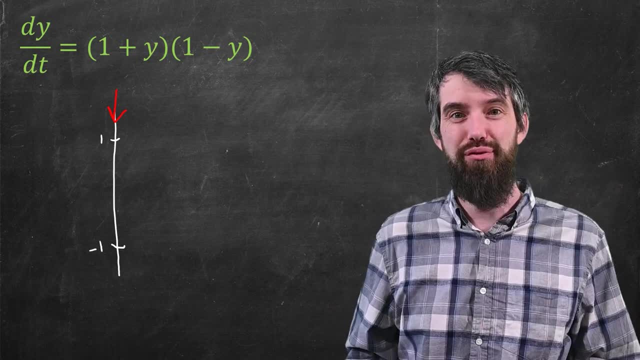 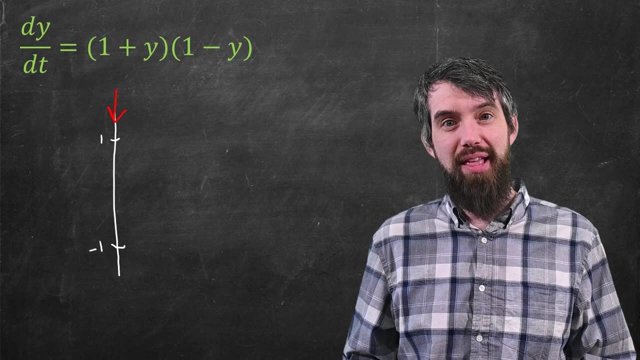 It's basically the same idea, It's just that we have this larger context of differential equations. Anyways, if I go in between the two equilibrium points, now say a value like y equal to zero- I plugged that in and that's gonna be positive. 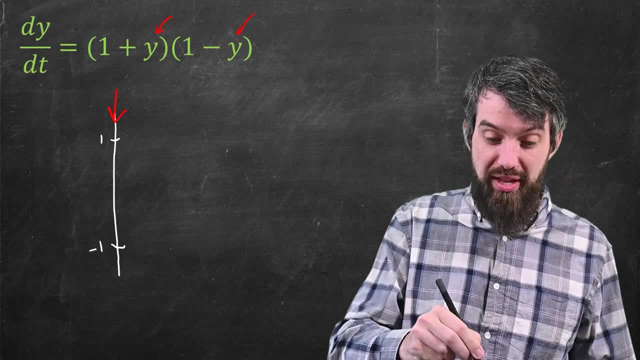 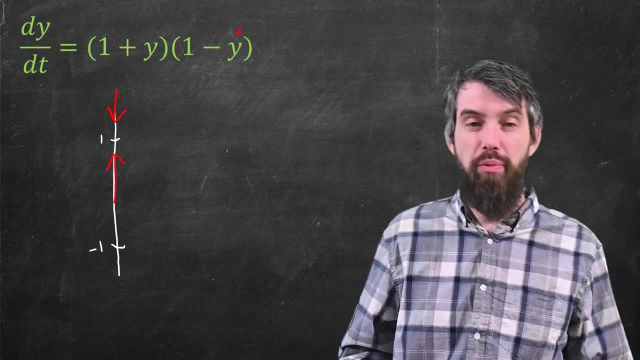 Right, Zero in for y there and zero in for y there, then this, indeed, would give you a positive value. So what I can deduce is that the arrow is going up in this middle portion, And this is what lets me conclude that the point which is y equal to one. 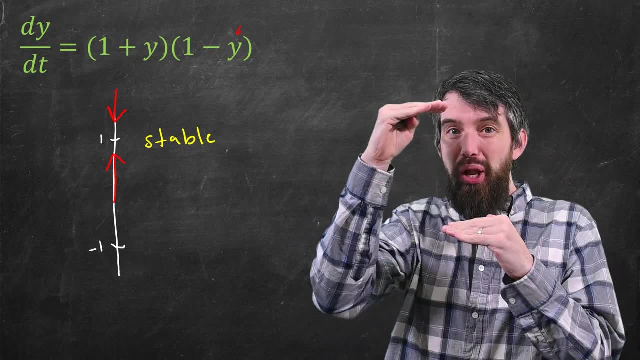 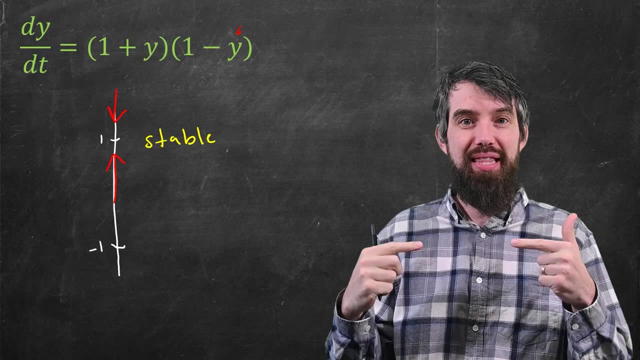 is a stable equilibrium point, because above and below the equilibrium point, the slopes are tending towards the equilibrium point. They're negative when you're above it and they're positive beneath it. We're just gonna send them to the equilibrium point. Finally, if you plugged in a number,